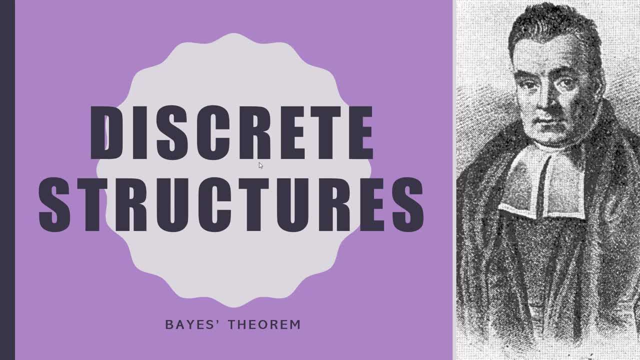 That little experiment we did with the beanbags. that is the very thing that he did, and I got the idea to do that from a Numberphile video. You guys ever watch Numberphile. To be honest, I'm not 100% sure it was a Numberphile video, but it was some of the same people. 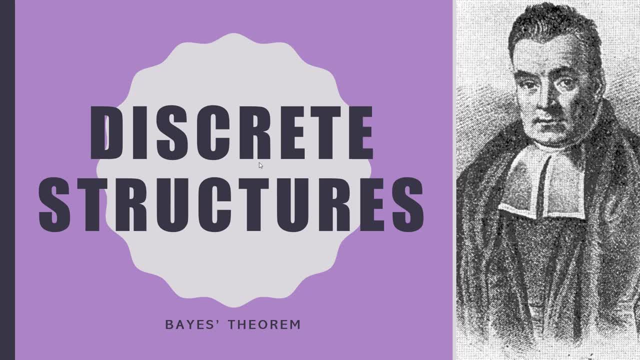 It was Hannah Fry and Matt Parker in the video. Hannah Fry, she's the red-headed girl that you've probably seen a lot of Numberphile videos, And then Matt Parker, he's the guy that does the stand-up comedy- math videos. 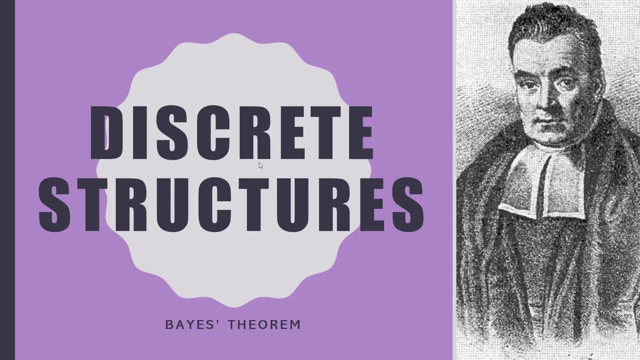 He has a stand-up comedy about spreadsheets. It's actually very hilarious. Is he a lanky guy or a curly-headed guy? Neither, I don't know, Matt. if you're listening, you may be lanky or curly-headed. I don't know which one that is. 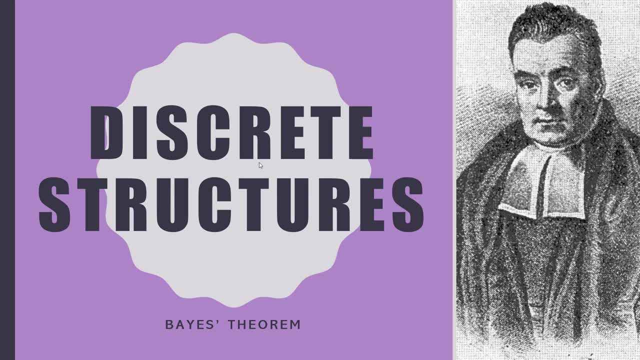 Not that he's ever going to see my videos. Anyway, they did the experiment. They actually did the experiment, the exact same one that Thomas Baze did, And so the idea again, as we talked about, is to update your understanding or your belief in something. 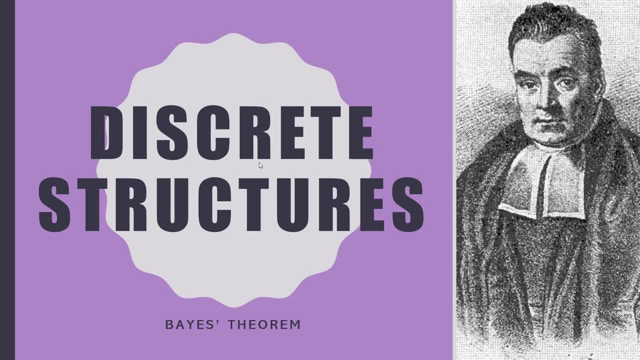 We all have a belief in different things, right? And that belief changes over the years, right? Maybe your belief in what is the best diet for you has changed over the years, right? I grew up My mom is from. I grew up from the South. 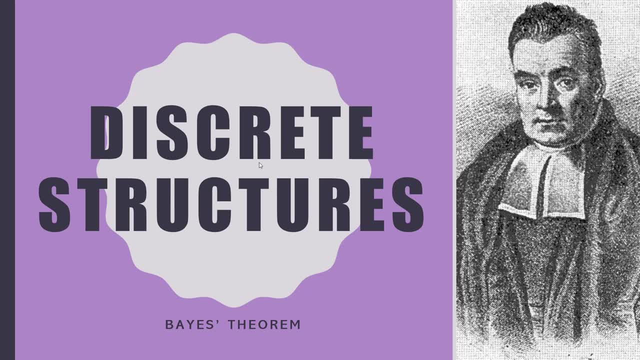 I grew up eating, you know, biscuits and gravy and fried food, And I just thought that's the way people ate. I believe that was the right kind of food to eat. Now, two decades later, and diabetes later, my belief in that diet has changed right. 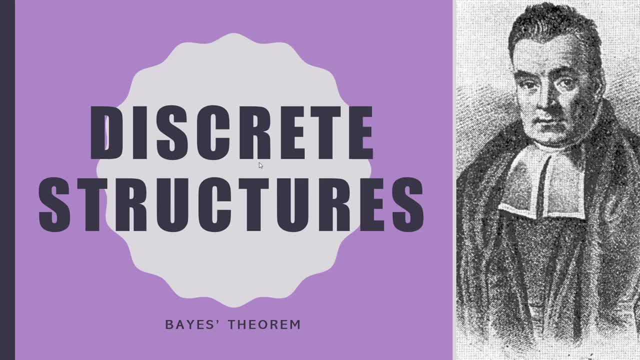 So now I've experimented with diet like the kid- And this is not a diet course, guys, But it fits into this Baze-ian idea. I've experimented with different types of ways of eating to control diabetes And I've had a lot of success with the keto diet, right. 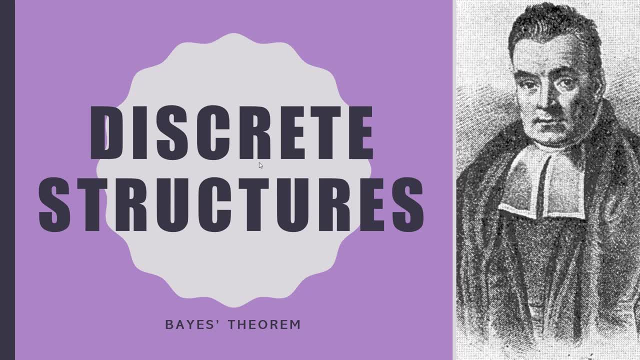 So hashtag: keto for life. What did you guys talk about in class today? Like serial killers and diets. It's all Baze-related Anyway, but I've updated my belief in the value of that kind of diet for me. It's been very effective for me. 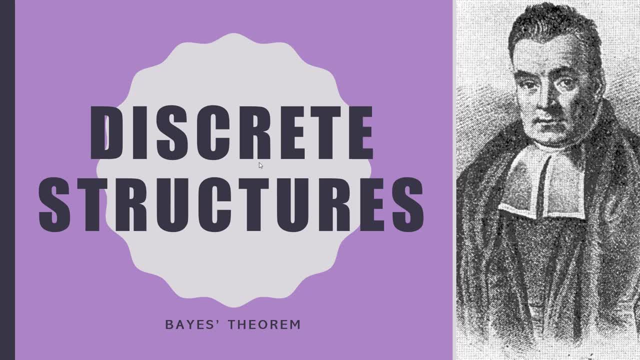 And so my belief has been updated. But it comes with things that can be plugged into a Baze formula right. It's hard to say that Baze's formula right, But it comes from From getting more data. The whole idea is: the more data you have, the more accurate you can be in your belief. 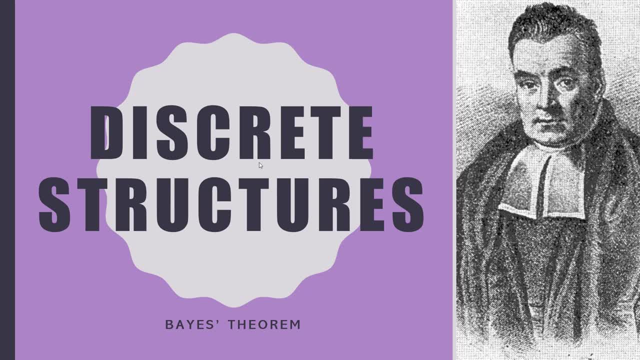 You'll never be 100%, though using Baze statistics anyway, There are some things that you can be 100% sure on right When you have all the proof and the evidence. But using Baze-ian logic and Baze-ian formula and statistics- whatever you want to call it- 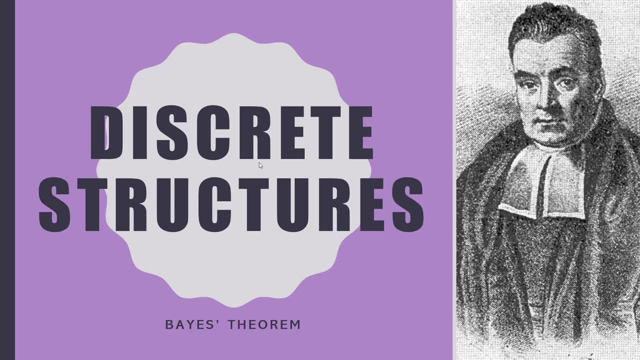 you can't be 100% sure, But this helps you hone in on it and get closer and closer to 100%. And, as with the beanbag experiments, and if you're watching this video and have no idea what we're talking about, 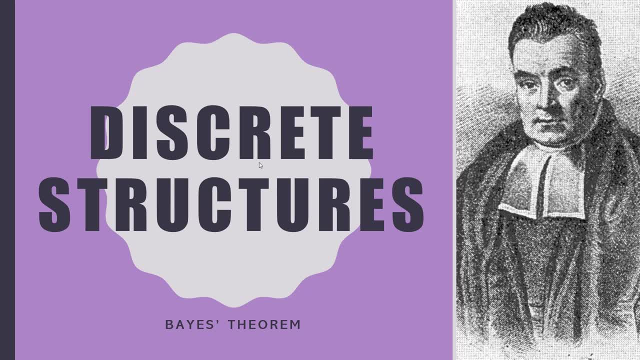 look in the video description There'll be a link to that beanbag experiment. But with that beanbag experiment, if there were an infinite number of beanbag tosses, eventually you could get almost 100% certain where that other beanbag was right. 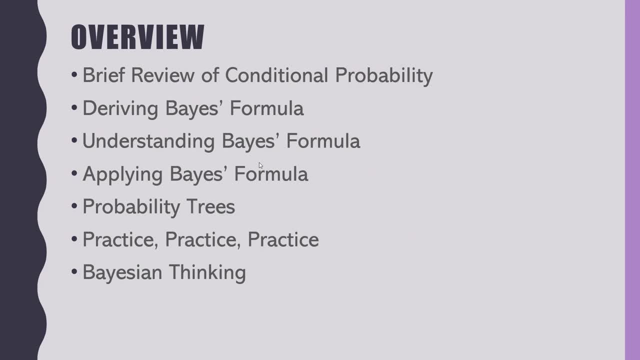 All right, so let's dive into this. Enough preface here We're going to do a brief review of conditional probability from the last couple lectures. right, We're going to see how Baze formula is derived from the conditional probability formula. 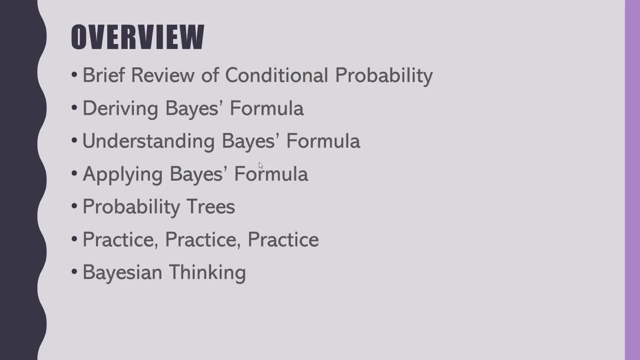 We're going to try to understand the formula, Then we're going to apply it, We're going to look at a probability tree: practice, practice, practice. And then we'll talk about Baze-ian thinking a little bit more, which is the stuff we've just been talking about, right. 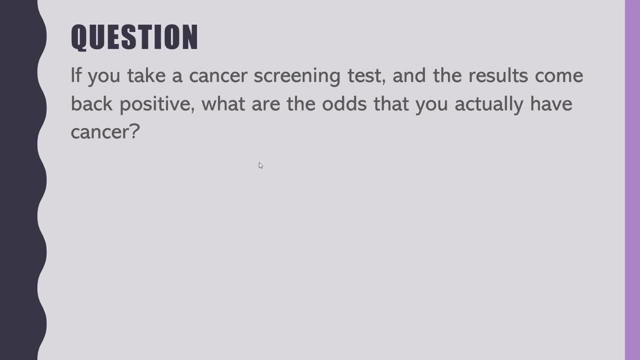 So I want to ask you this question first, And I'm not going to give you the answer right now, But I want to just sort of take sort of a- what's the word an? informal poll. right, If you take a cancer screening test, and specifically the cancer test we're looking at is breast cancer, 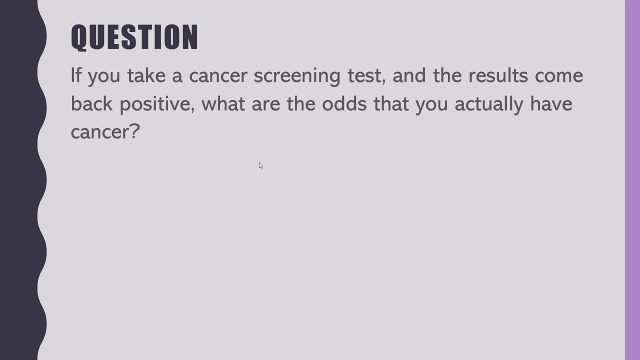 for women between the ages of 40. And 50, that's the specific one we're talking about. If you take a cancer screening test and the results come back positive, what is the probability or what are the odds that you actually have cancer? 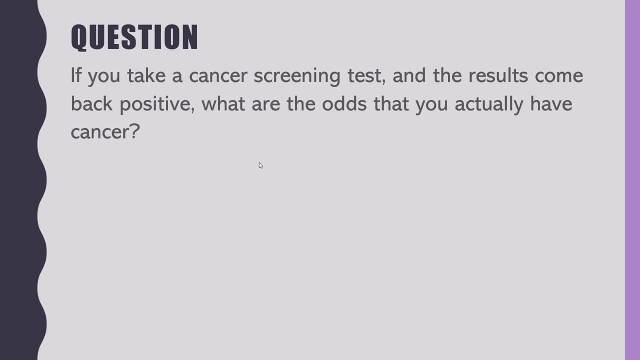 Okay Now I don't expect you to know that Some of you may be familiar with this idea, But just, I'm going to write on the whiteboard here And maybe I'll do an overlay on the computer here to show the numbers we came up with. 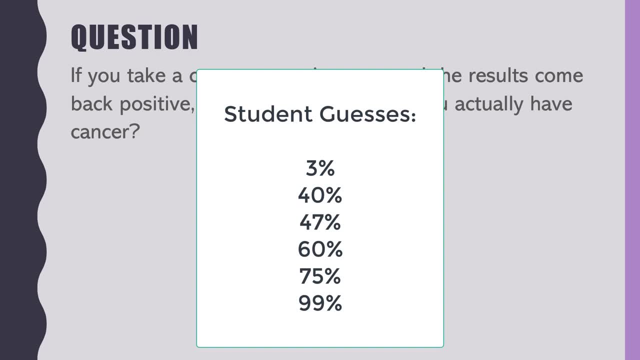 So I have to pull in the class. We've got a few numbers here that you should be seeing on your screen right now. You'll see there's a wide variety of them there. We will answer the question At the end of the lecture. 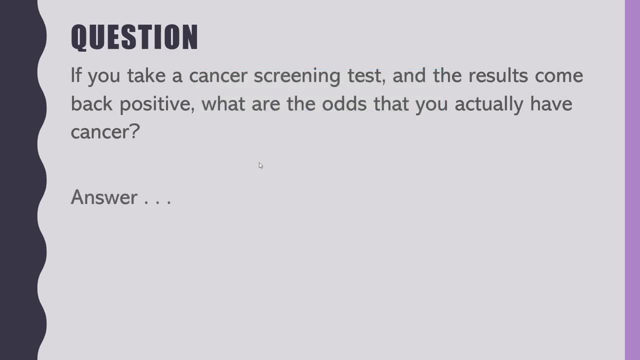 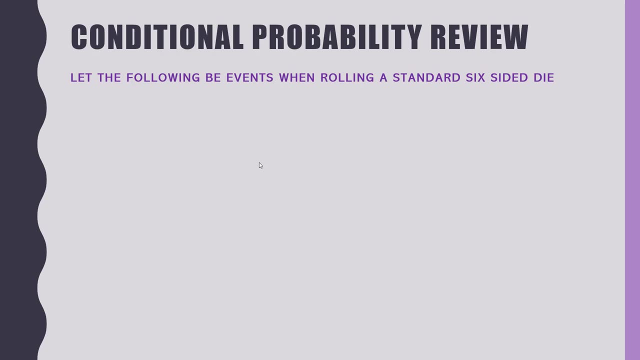 So stand by and stay awake. Answer: just told you end of the lecture. All right, So here we go. Review of conditional probability. We're going to do this very quickly. You guys should know these. Let the following be events when rolling a standard six-sided die: 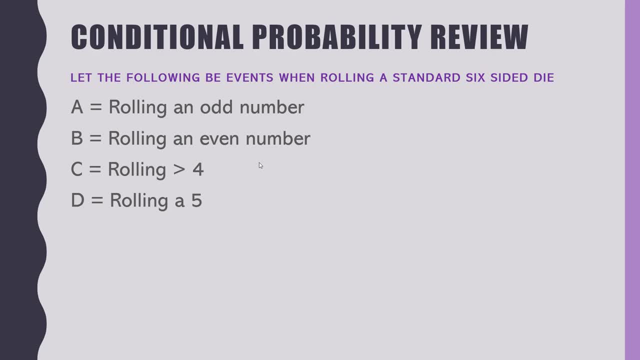 A is you're rolling an odd number. B, you're rolling an even number. C, you're rolling a number greater than four. And then D, you're rolling a five. All right, Without even having to use the formula, we're going to do this. 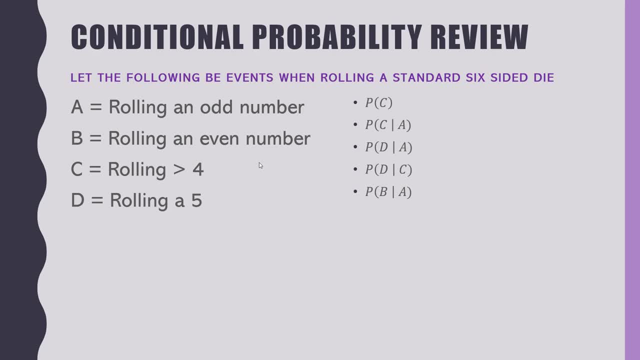 Okay, We can answer these questions pretty easily, because the sample sizes are very small. What is the probability of C? Right, You're correct, It is one-third. Let's speak in terms of the actual size of the sample set, though. 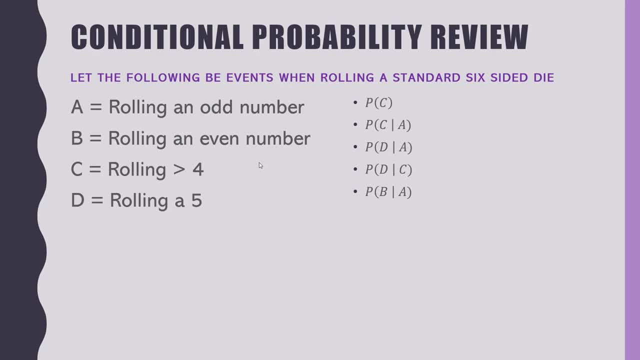 So what would that be? Two out of six, right, And yeah, of course you would want to reduce that down, But I just want to make sure that we're all on the same page. So it's two out of six is your probability. 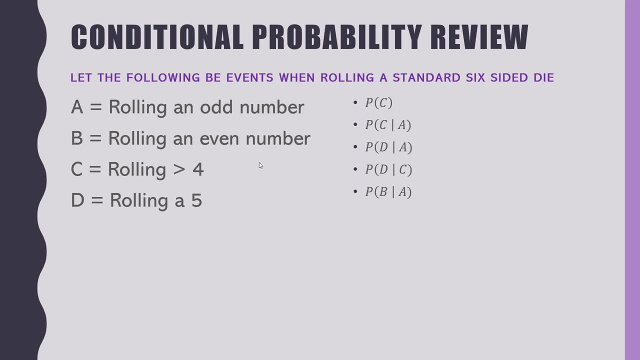 All right. Probability of C given A. So what the question is saying? what's the probability that you're going to roll something bigger than a four, given that you did roll an odd number? One-sixth, No, one-third? 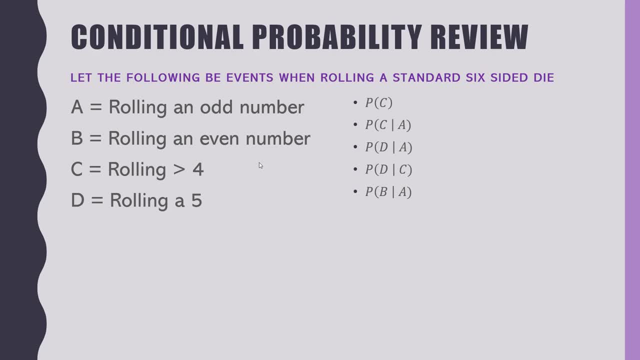 Sorry, you're right, It is one-third. Yeah, Don't listen to anything I say, I don't know what I'm talking about. One-third is correct. Why? Because our sample set is now one, three, five. Only one of those is greater than four. 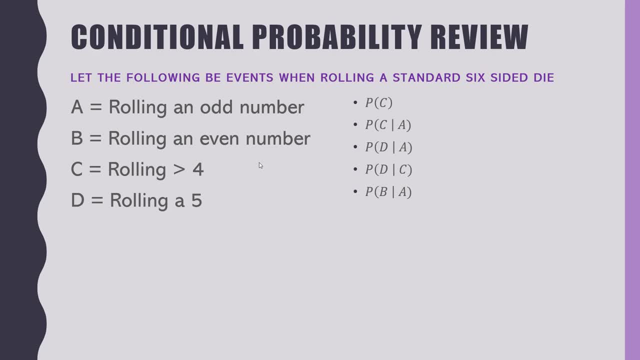 Right, Good, Okay, Probability of D given A. Probability that I rolled a five, given that I rolled an odd number. Yeah, that's the exact same question as the one right before it: Probability of C given A. I'm essentially saying: 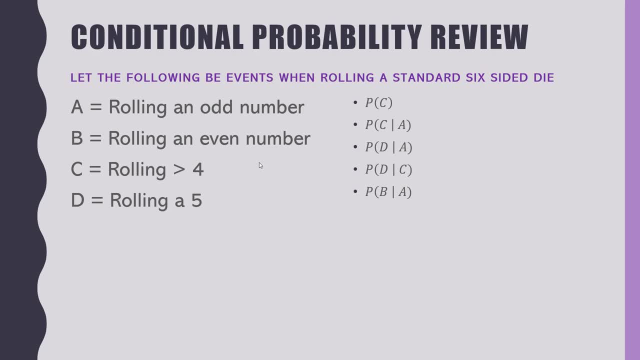 what's the probability of me rolling a five? That's the only odd number greater than four, Right? So those are the same: Probability of D given C. So probability of rolling a five, given that I rolled greater than four. Yeah, sorry. 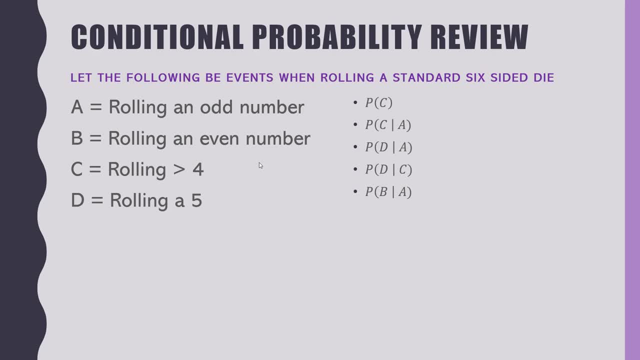 One-half right Probability of rolling a five, given that the number is greater than four. Well, if the number is greater than four, that's the given. What's our sample set? Just two things right: Five and six. 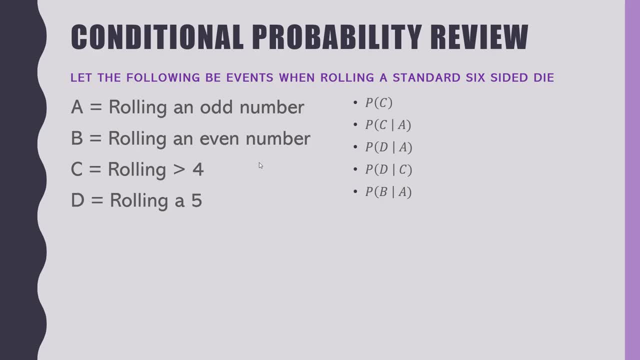 One of those is a five, So it's one out of two shots, right, And I'm going to put the numbers on the screen in a moment. And then the last one: probability of B: given A Zero, right, The probability of me rolling an even number. 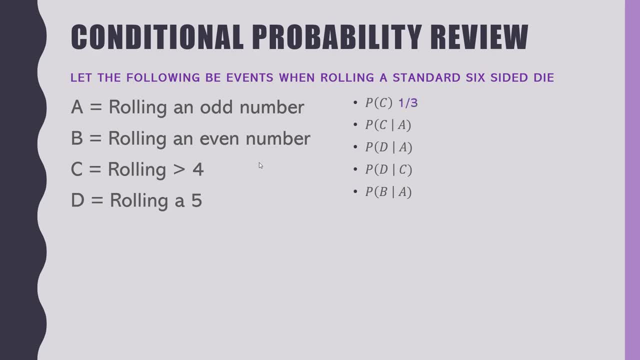 given that I rolled an odd number, Obviously that's zero. Okay, Okay, And these are the answers here. We probably should have been playing them as we went along. Okay, Look at those. Make sure you understand why those are all true. 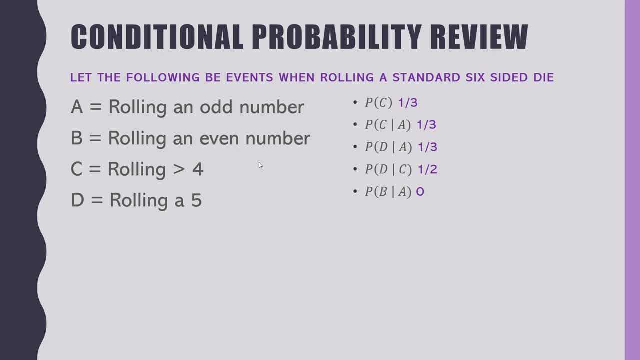 We understand them. Okay, This is the review part. We should be familiar with this, But if we're unclear I want to make sure We good. Okay, let's take a look at a couple more here. Let these be the events when drawing a card from a deck of cards. 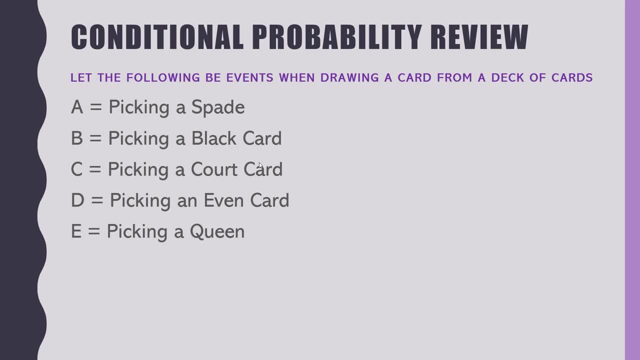 You picked a spade, or you picked a black card, you picked a court card, you picked an even card, you picked a queen. So what is the probability of each of these These events? Probability of A given B, So probability of it being a spade. 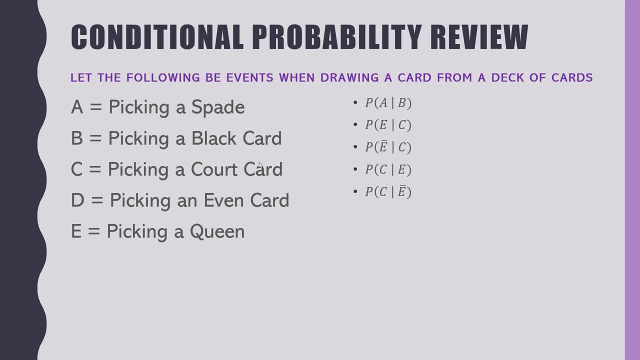 given that you picked a black card. Now you have to be familiar with the deck of cards to answer these. I'm assuming most of us are. But just in case right, there are 26 reds, 26 blacks. The black cards are 13 clubs, 13 spades. 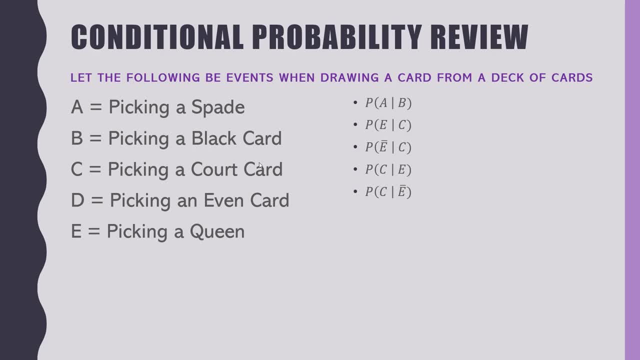 Red cards, 13 diamonds, 13 hearts, right. So what is the probability of A given B, One half, And what's the original numbers? We would have there? 13 over 26, right, Which is one half. 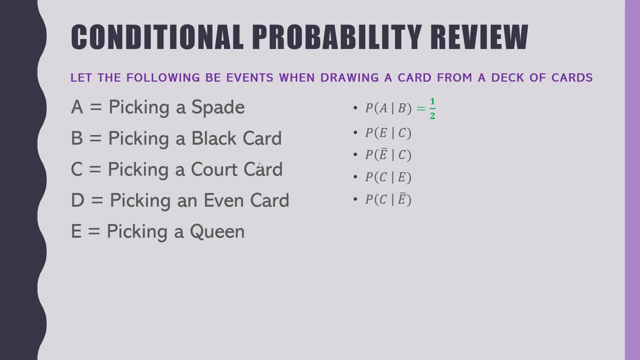 Very good, Okay, Right. So 13 little spades. You have 13 spades to choose from And we know we picked a black card, which means our sample set is 26.. All right, Probability of E given C. 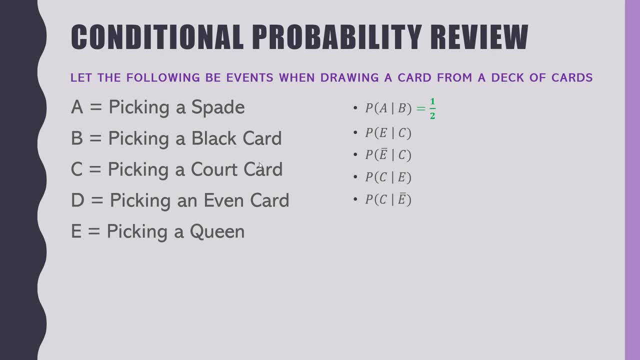 Picking a queen, given that we picked a court card. Courts are jack, queens and kings. Four, twelves, Yeah, very good, Or one-third exactly what you just said. You looked at my slide in ahead of time. 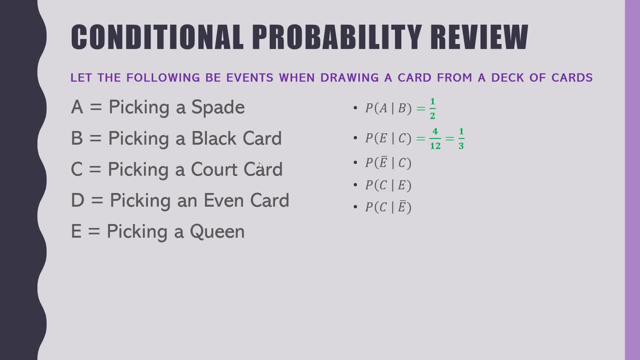 Good, All right. What is the probability of not picking a queen, given that I picked a court card? Eight out of 12, right, Which is two-thirds, Make sense. If any of these numbers are unclear, stop me and we'll make sure we understand them, okay. 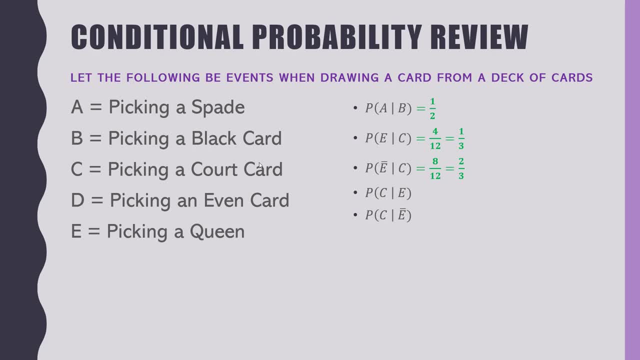 Next one: Probability of picking a court card. given that I picked a queen- One-hundred percent right, Because I know it's a queen- What's the probability that a queen is a court card? It is always a court card, right. 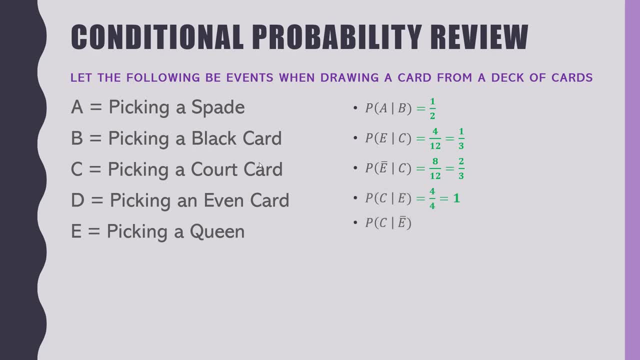 Very good. One-hundred percent, Four out of four, right, And let's make sure we understand that four out of four. Probability of it being a court card, given that it's a queen. Well, if it's, given that it's a queen. 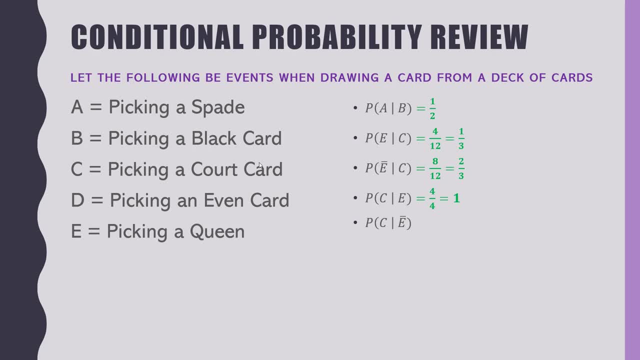 assuming this is a normal deck. there's four. That's your sample set, And what's the probability of me picking a queen when I've only got four? There's four chances I can pick a queen, So it's 100%. All right, last one. 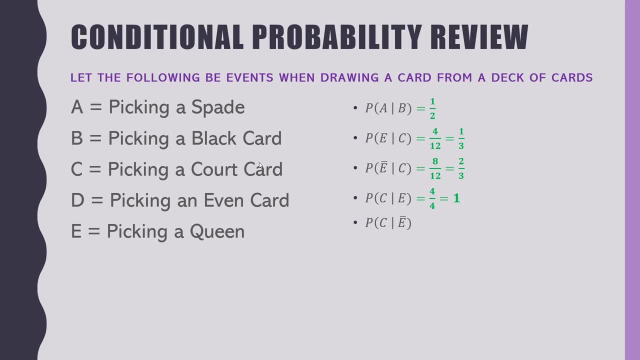 Probability of picking a court card, given that it is not a queen, Very good, Eight out of 48.. You see why, Right, It's not a queen. so that eliminates four cards from the deck. The deck's 52,, right. 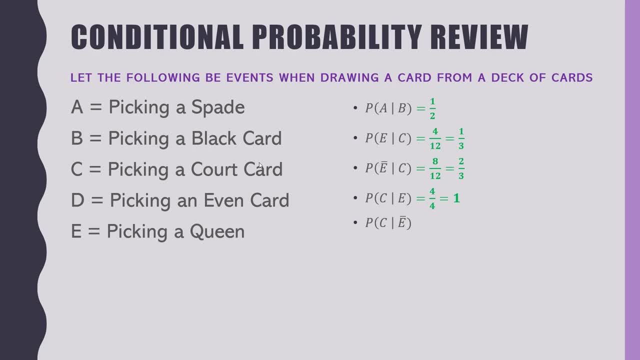 You minus out the four queens, you've got 48.. That's your new sample set, Given that, it's not a queen here, right? So this was the given It's not a queen, Given that sample set of 48,. 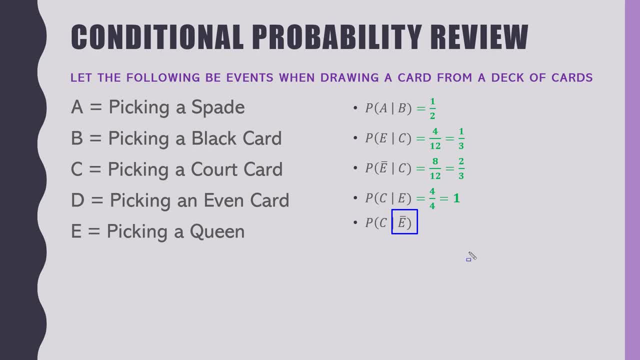 what's the probability that I'll pick a court card? Well, there's only eight cards left in that deck of 48 that are not queens right, Or that are court cards, I should say, Which does give us eight out of 48, which is one-sixth. 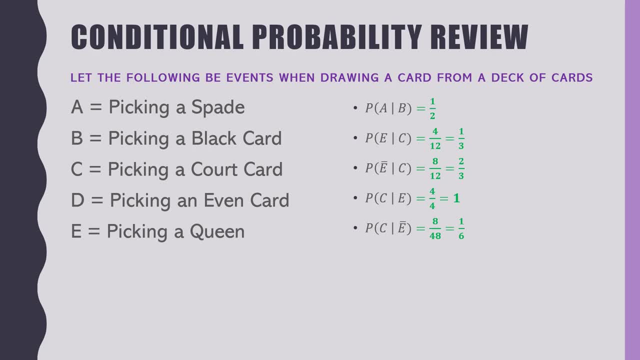 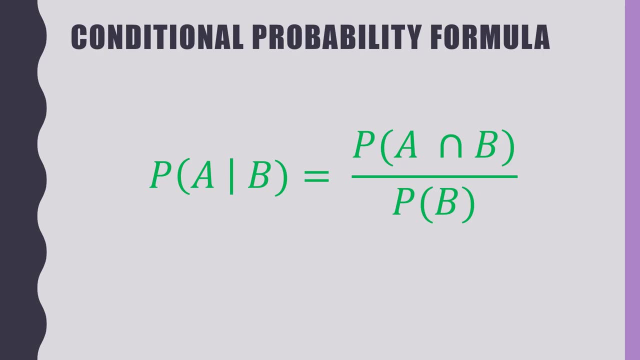 All right, That's the review portion. We feel okay about that. Let's remind ourselves how the equation works. This is the probability equation, right, And we're going to look at two Venn diagrams here to help. Again, this is all memory-triggering, hopefully. 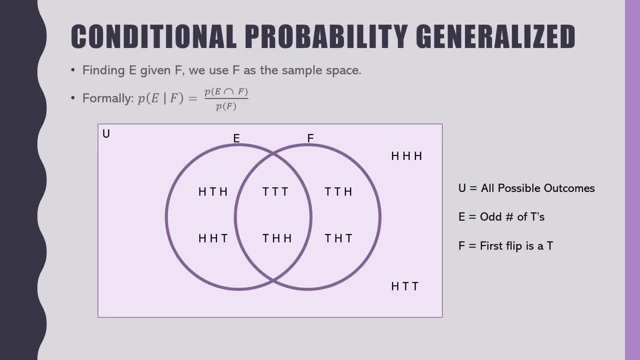 to remind us of what we talked about last week. We had this exact slide last time, right? So just briefly, let's look at this: The universe is the whole lavender box and it's all possible flips of a set of three flips, right? 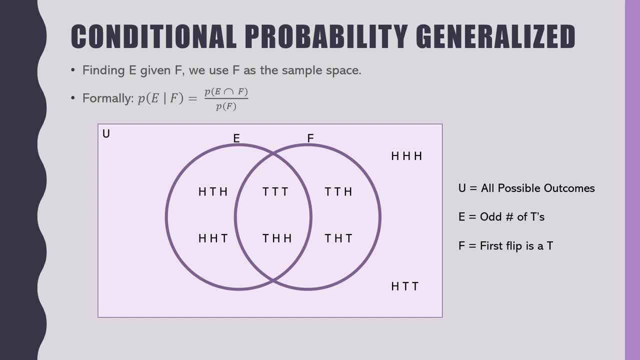 I flipped the coin three times. There's only one: two, three, four, five, six, seven, eight ways that that can pan out right. You can see all eight ways that I can get three flips right there, assuming there's only a head and tails. 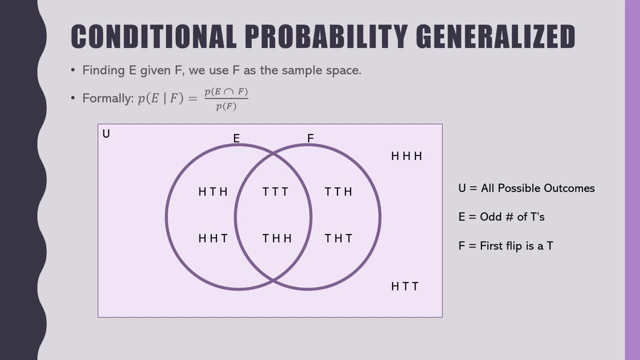 there's not going to land on the edge, right? Okay, Then you see that E is the number of flips that have an odd number of tails, right? The E in the Venn diagram and then F is where the first flip was a T. 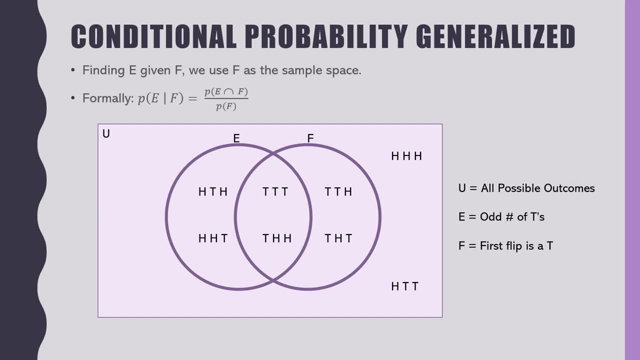 If you remember, the question was: what's the probability of us having an odd number of tails, given that the first flip was a tail? Well, where is that on the Venn diagram? That's the intersection. That's the intersection. right there, right. 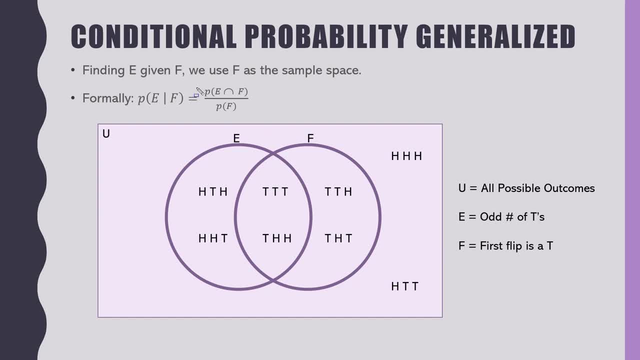 Okay, That's where we get this formula. It's this divided by this right, Because the F is this stuff right here- that the first flip is a T, a tail, And I'm asking: what is the probability of this? 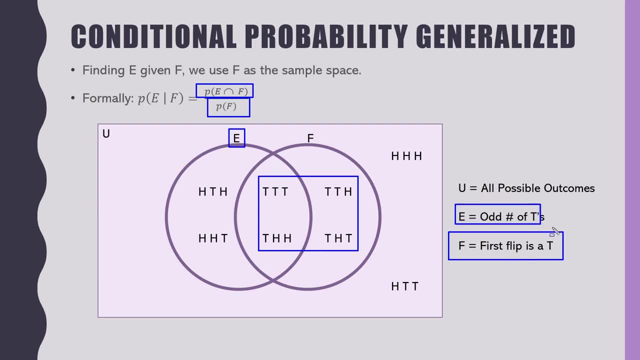 of E happening. and what is E? It's an odd number of tails, given that F did happen, right, Given that F happened. That's what that piece means. Well, it's the probability of that intersection which is right, with the probability of this happening. 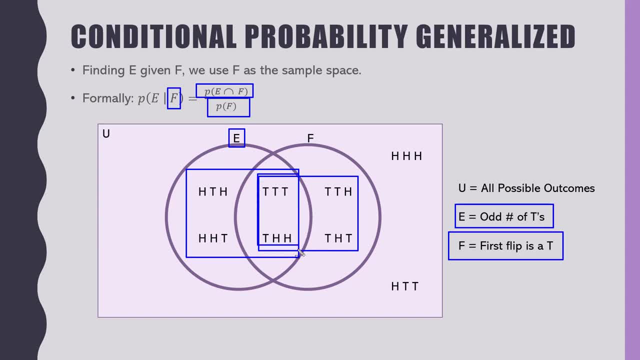 given that that happened, The answer is this: divided by this, That make sense. Okay, let's look at it with the playing cards, because that's the same example we just saw a second ago. All right, This is an entire deck of cards right here. 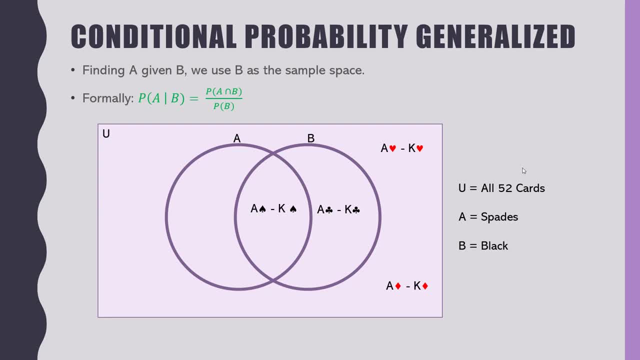 I didn't want to make a single ace and two and three, so I just did ace through king, right, But this is the entire deck. This is the entire deck of cards. Now, the universe is all 52 cards. We're leaving out the jokers. 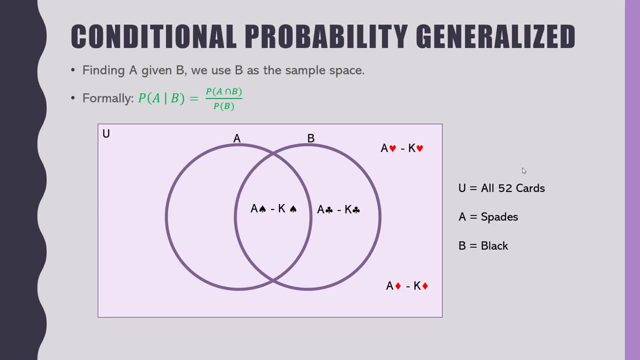 A is that it's a spade. B is that it is black. The red ones are neither of those things, right? So our question a minute ago was: what's the probability that it would be a spade, given that it's black, right? 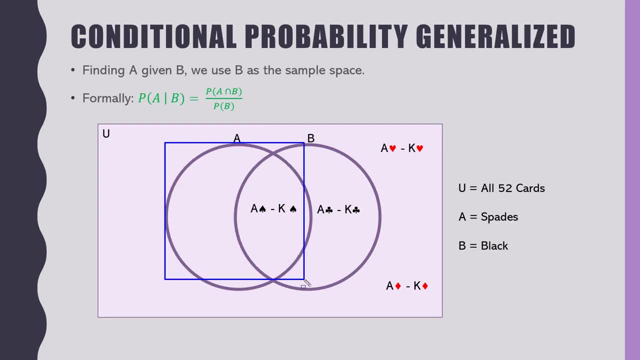 So what is the probability that it will be in this circle A, given that we know 100% sure that it is black in B? right notice, when I draw my little blue lines I end up with that intersection again, that's the those blue lines are making their own Venn diagram. 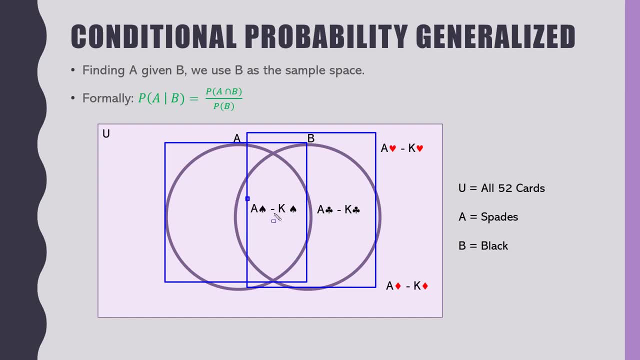 just squares instead of circles. so, in other words, it's this number divided by that number. well, this number is the intersection of a and B, and this number is B, or the probability of that intersection divided by the probability of that intersection of that. that's it make sense, that's the formula, that's. 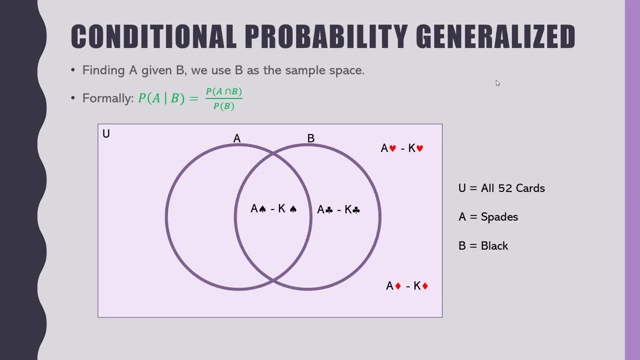 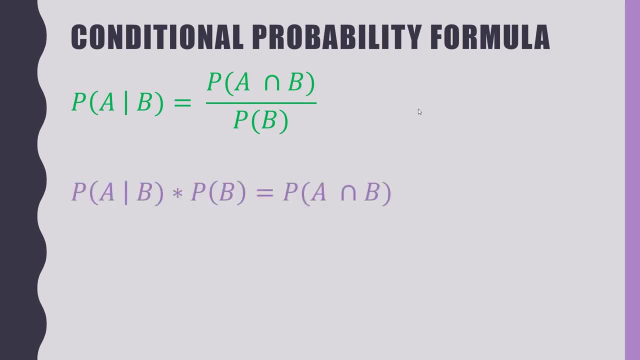 what we talked about last week. hopefully that's pretty clear. that's a review, because? but this is the foundation of Bayes theorem. okay, so here's that formula one last time here now. would you agree that that is the same thing, just algebraically, algebraically, right? 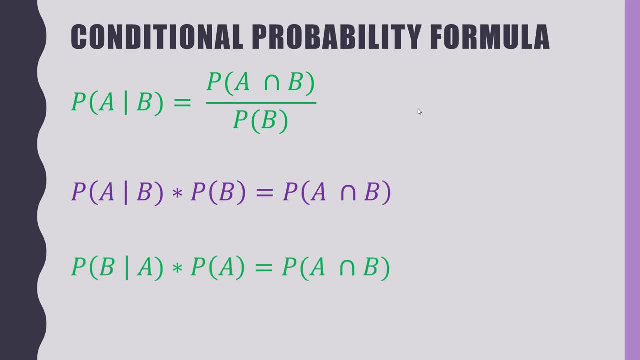 would you agree that that's also the same thing? now take a minute and look at this one. okay, the part that throws people off here sometimes is this: I'm saying the probability of A given B times the probability of B is the probability of the intersection. remember that the probability of the 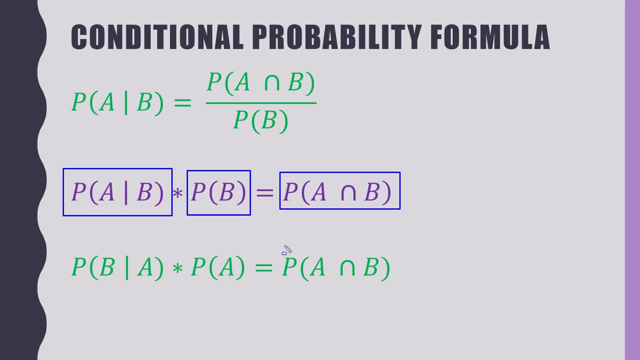 intersection of A and B is the same thing as the probability of the intersection of B and A, right? the order of the A and the B when you're dealing with intersection is irrelevant, so I'm keeping in the same order there, right? I could have, if I wanted to, to make it seem a little more clear, reverse the A. 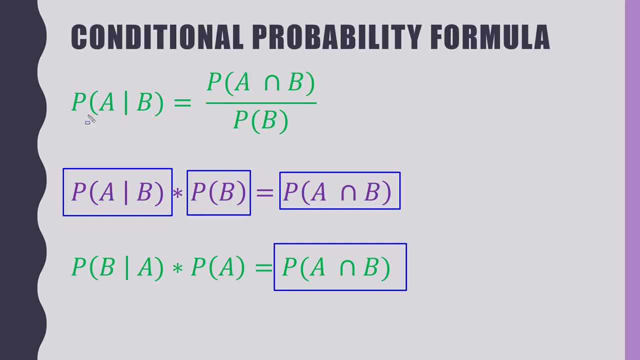 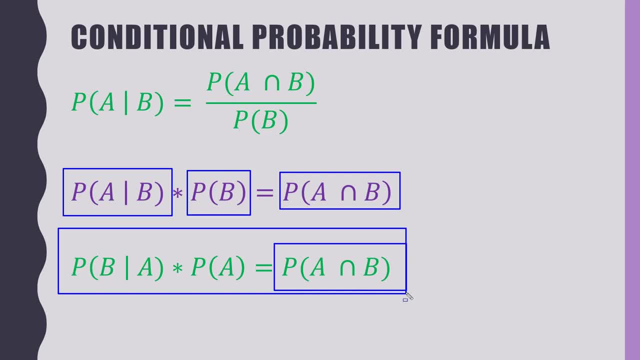 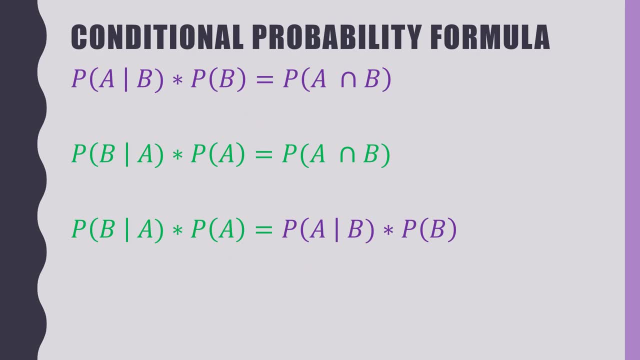 same argument is the two ways that our formula isisesti put right. so this formula: we agree that both of these formulas are correct and accurate. all right, because I'm gonna race the top one in a minute. I'm gonna make sure we buy into this, okay, all right. so everything on the screen here. now look. 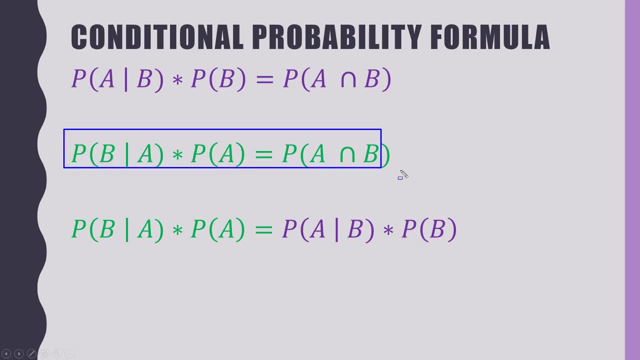 at that. third one. would you agree at that statement? all we did here is still kept this piece of it right here. then we would just replace this with this value, which came from this formula. agreed, all right, so here's that formula again. we're just going to keep that front center for a moment and we're 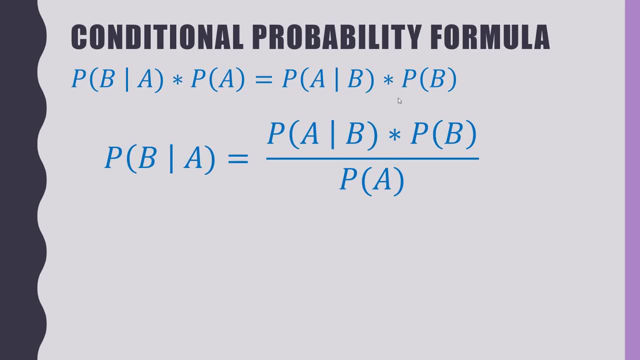 going to change the color to make it fancy. okay, would you also agree that that's true? just algebraically rearranging stuff here, that's all I'm doing: a little bit of substitution, some algebraic rearrangement. the probability of B given a is equal to the probability of a given B times the probability of B. 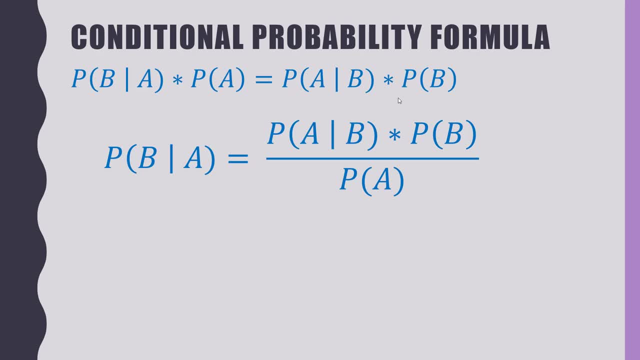 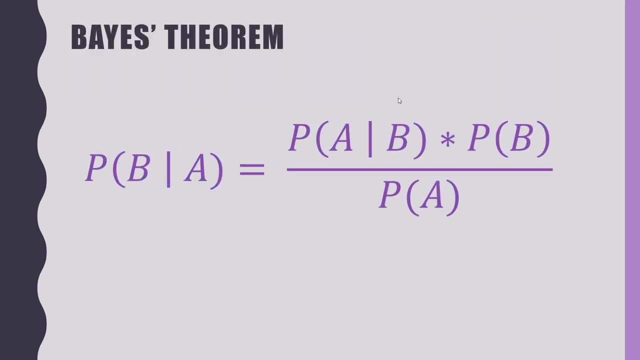 divided by the probability of a. that's Bayes formula. right there, okay, we're gonna see how it applies, but there's one extra piece we need to account for. okay, okay, okay. the last thing we need to take a look at here is this: right here, getting the. 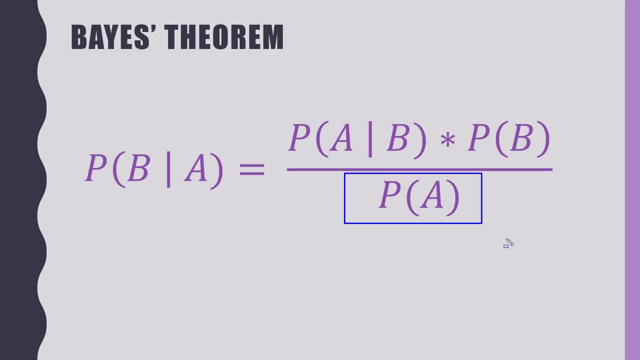 probability of a given B and the probability of B. usually those are easy things and will just be known facts or whatever. but what is the probability of a in whatever question we're trying to answer? that gets a little tricky that we have to deal with total probability and we're gonna look at some probability. 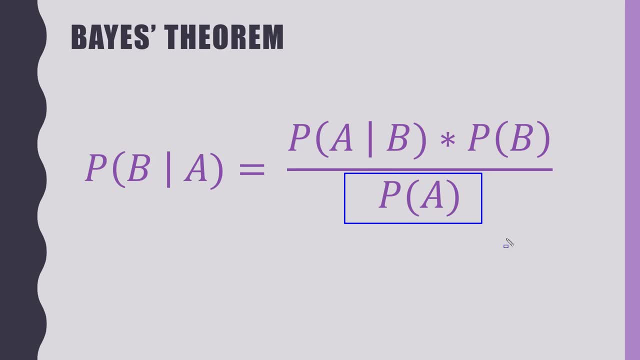 trees and some ways to figure that stuff out as we move along. but the normally the top part of the equation, the numerator, is pretty much stuff that will be given or, with the data we have, it's easy to figure out. calculating the denominator gets a little trickier. all right, if you remember when I first introduced you to. 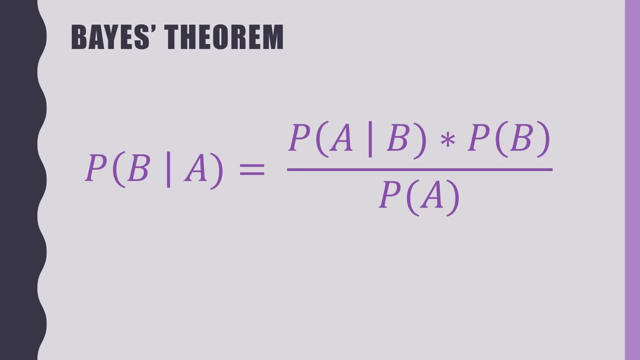 probability. what did I say? it's just favorable outcomes over possible outcomes, right? or we now we use the more formal terminology, which is events over sample space, right? well, and I also said that that's easy, right, it's something divided by something. that's an easy thing to calculate. what's hard is 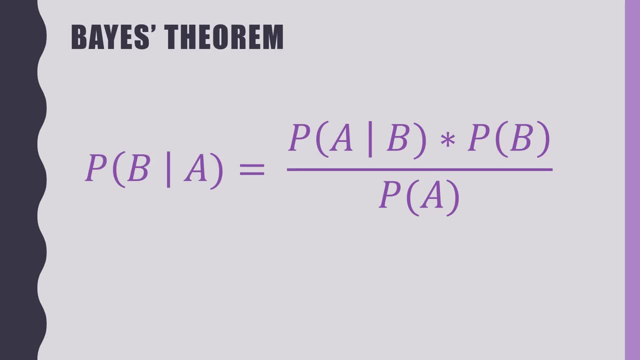 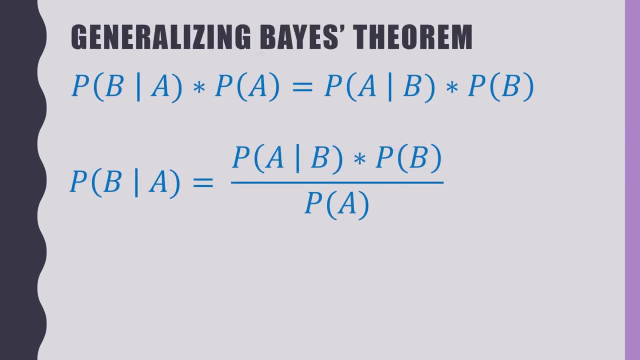 figuring out what is the E, what is the S? and now I've made it even harder, right, because we're expanding this, okay, but it's still the same thing. it's something divided by something. that's what probability is. so let's sort of generalize this just a little bit here. all right, we've got these two, the 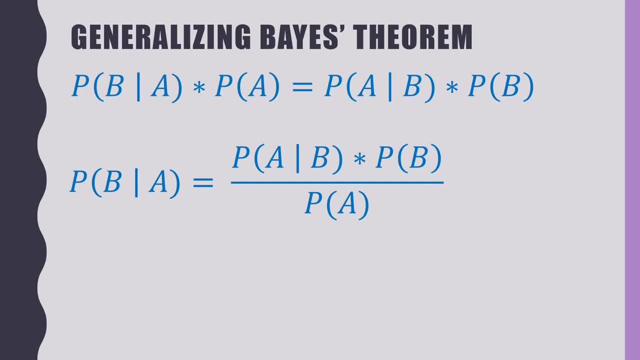 they're the same equation here. we just rearranged them in one case, but we're gonna do a little bit of playing around here, okay? so let's take a look at a Venn diagram first. this is just some universe of some events, right? I don't know what the events are, doesn't really matter, we're just gonna. 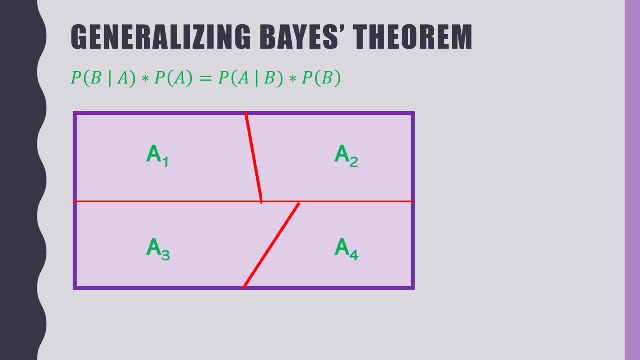 be general here and I'm going to, our Venn diagram shows event a1, event a2, a3 and a4. notice here that all four of those events, if they, if you add them all up, you get the entire universe based on this Venn diagram. right, most of our Venn. 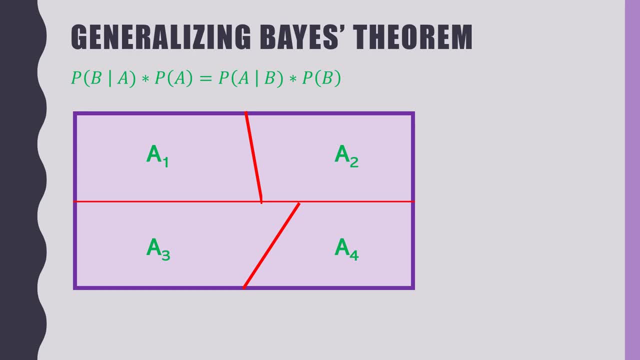 diagrams. we got the two circles in the middle and there's still a whole universe where there's stuff that isn't necessarily in our events. but we're gonna take those in our events and look at them in that straight line. but here I'm saying that event one, two, three and four, if you add them all up it is the entire. 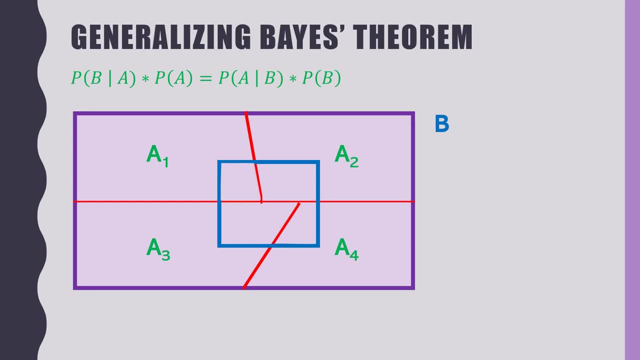 universe agree. okay, now we have another event called B. okay, this event occurred. this event is not the entire universe agreed. I want some nods on this stuff to make sure we're we're good on this, because it's it's gonna get a little more tricky as we move along that yellow section right there. how could we? 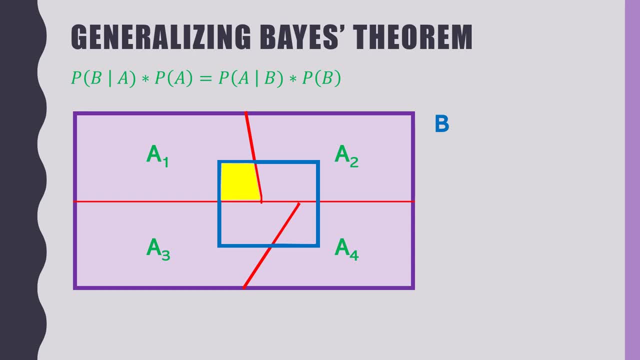 what is that? the intersection of b and a1. very good, right? everybody see that. the intersection of a and b1. okay, now you know that. i think the next one should be pretty easy. how about that dark blue? what is that? yep, a2 and b, right, okay. and then obviously the next ones, though each of those sections, do you? 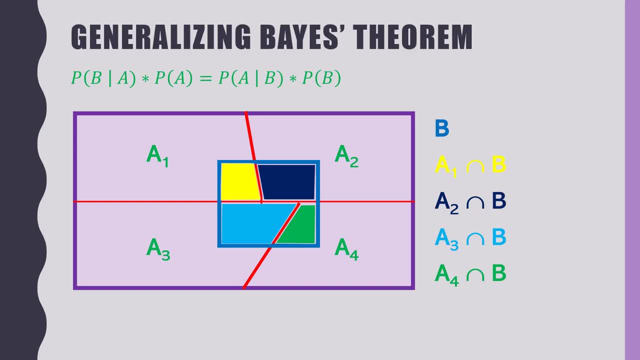 agree with those pictures. i tried to color code them and this thing's going to get pretty colorful and get a little messy. but do we agree with everything on the screen? do we understand it? okay, and i apologize for asking that question a thousand times, but i want to make sure that, as we 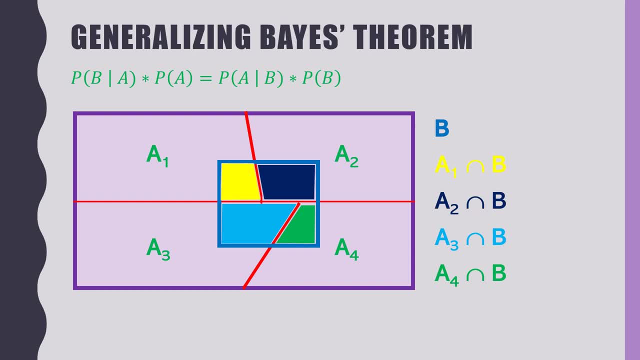 move along and we get to the final base formula that you just believe in it, right, i'm trying to update your belief in base theorem, okay, all right, there's a little self-referential humor in there, yeah, um, so the entire universe in this case is a1, a2, a3, a4. 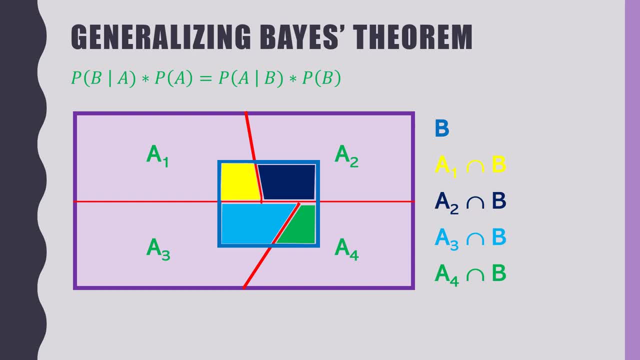 added together. yeah, yep, exactly, right now we could. if we had an expanded universe that was bigger than that purple lavender thing, then maybe we might see that that a1 box finally closes in and there's some stuff outside of the a1 box, but this particular thing. so take, for example, 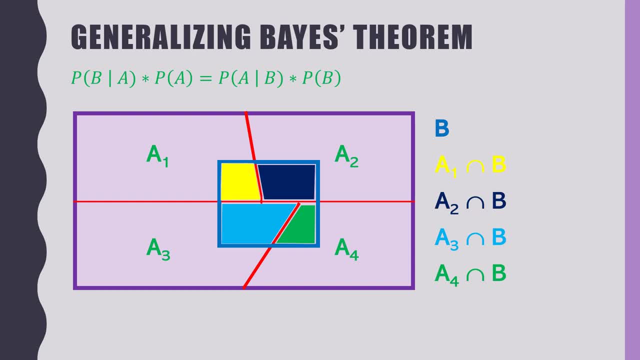 the idea of a universe of flipping a coin: heads and tails. i can split that venn diagram right down the middle and one side's heads, one side's tails and that is the entire universe. right, that that term for this is, and i think it comes up on a slide in a minute. 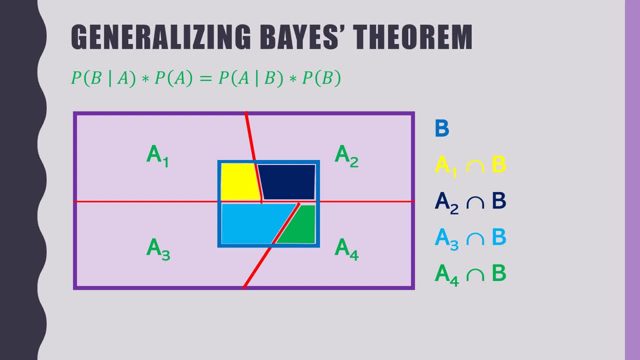 is mutually exclusive and, um, collectively exhaustive. that word collectively slip my mind. mutually exclusive, collective, collectively exhaustive. so what i mean by that? think about again the heads and tails. if you get a head, you didn't get a tail right. they're mutually exclusive events. you can't get both right. i cannot get a1 and a2. 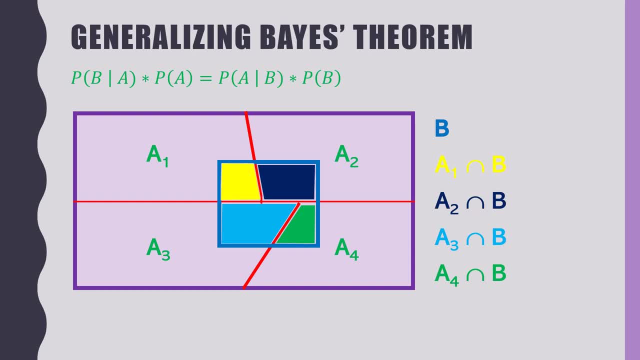 right. they're mutually exclusive. they're collectively, collectively exhaustive, because if i get a head or a tail, that's the entire universe. there's no other part of the universe. so whatever a1 is- again i'm trying to generalize here- so a1, who knows what? that is right, but it's. 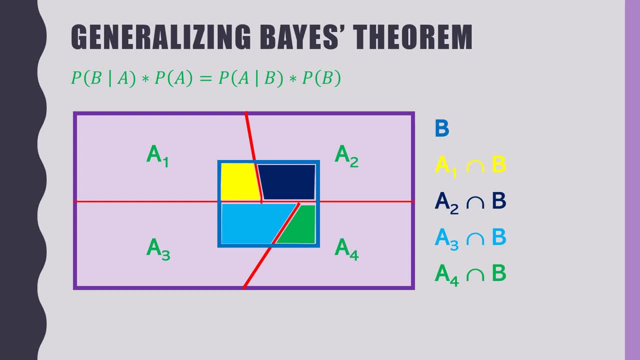 a1 and a2 and a3 and a4 is the whole universe. okay, good, good question. so now we got b and we can define b as a whole universe. so we can define b as a whole universe. so we can define b as a whole universe. 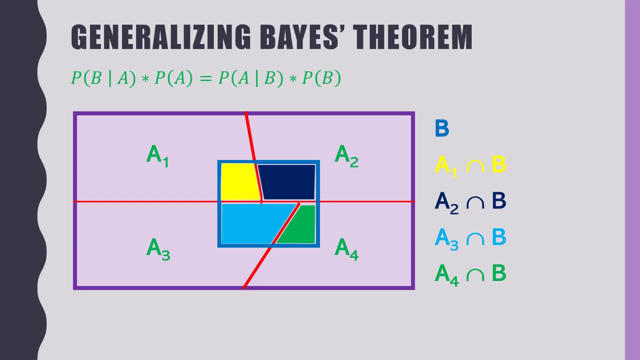 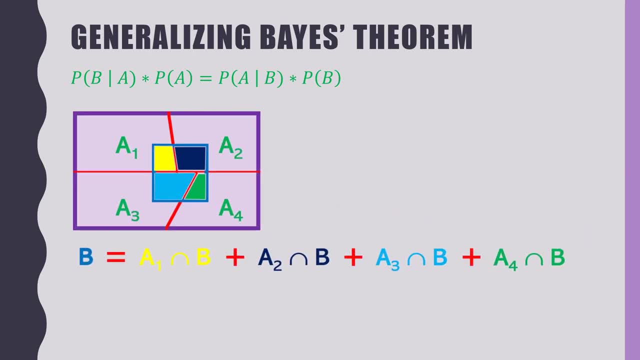 as the intersection of itself and these other pieces of the universe agreed. and those four little things on the right there. would you agree that b is equal to the intersection of one and b the intersection of two and b. right, would you agree with that formula on the screen? 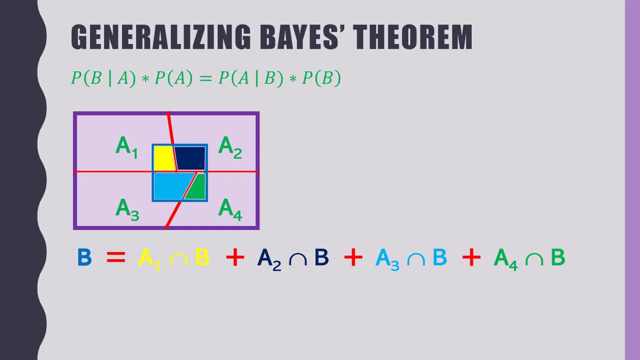 makes perfect sense, right, all right. if that's the case, then, and there's, i told you those terms are going to come up. we understand those two terms there. need to explain those again. yeah, is there a universe subscript? so you did a subscript u. is that how you define a whole universe like? how do you do that mathematically? 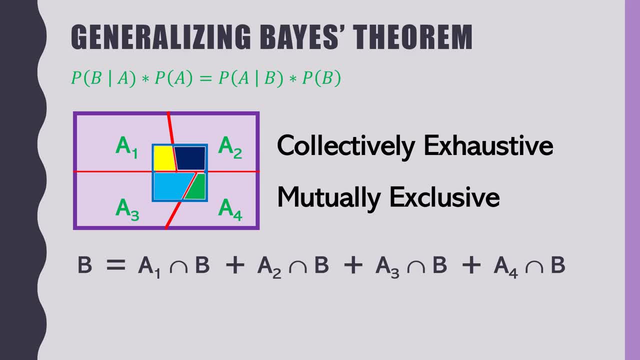 a universe. well, so you're asking how they define a universe. well, yeah, if you're talking about a universe, you can use whatever variable you want, but typically they will use a u. okay, yeah, so the universe, in this case u, is equal to a1 plus a2 plus a3 plus a4, correct? yeah, yep, all right. other 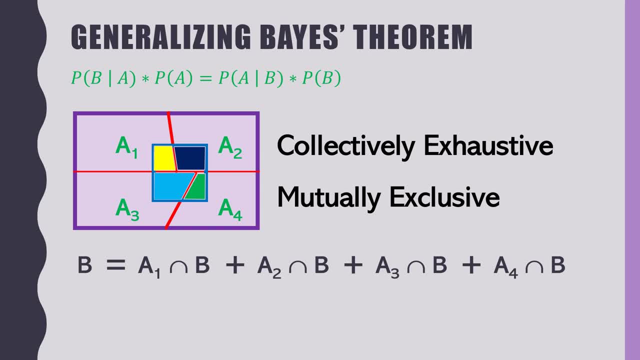 we're going to add a piece to it. so i want to make sure we're good. if that stuff in black there is true, then isn't the stuff in blue there also true? the probability of b happening is whatever: the probability of yellow happening plus the probability of dark blue happening, plus the probability of that green plus the probability 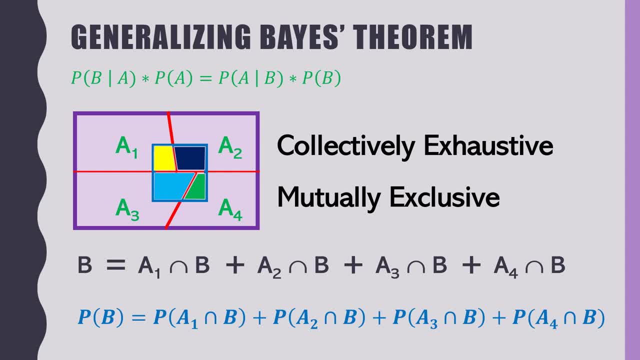 of that light blue happening. do you agree with that? yeah, everybody. yeah, okay, questions about that. all right, now it's going to get crazy crazier here. okay, i just want to make sure baby steps along the way, so we're going to take that formula that we 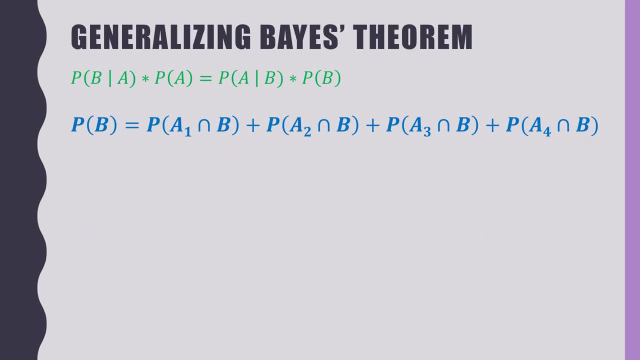 all agree with that. venn diagram helped us derive this using stuff we already know and remember this formula here. okay, this is our original probability formula. okay, probability b, given a times probability of a, equals intersection, which is that's which we. we know this to be true. we looked at it in a previous slide. okay, 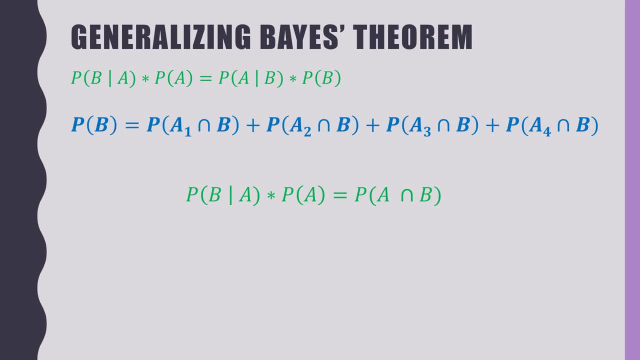 so we're good so far. just, i just want to remind us of what these formulas are, because we're about to do some substitution here. it's going to get a little messy. all right, that term, right there. the probability of something intersecting the other thing, or that, or that, or that. 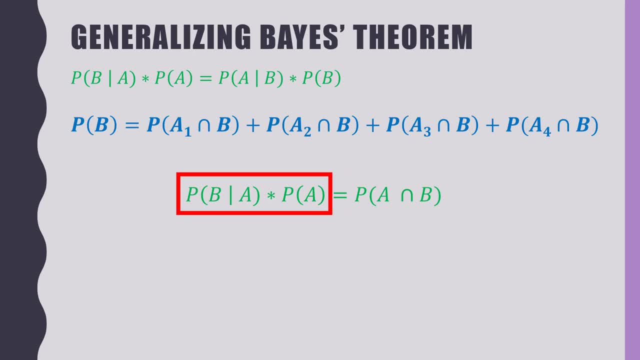 you agree could be written that way, because what i have here is the probability of a intersect b. well, i have a bunch of a intersects b. i have the probability of that one and that one and this one and so on. well, i could substitute this for this. it's the same thing, agreed. why, jeff? why are we doing this? i promise we. 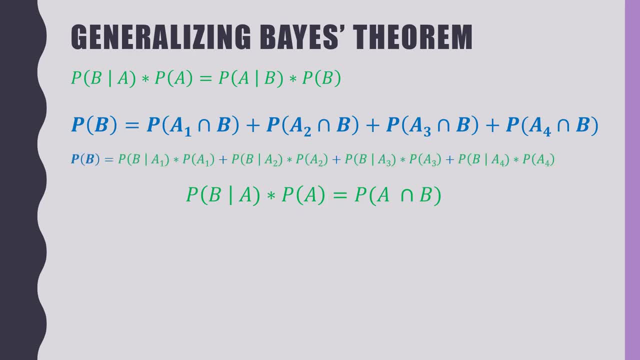 have purpose. so now i've rewritten that stuff in blue above to that new equation. that's kind of smaller there, assuming i didn't make any typos and using this as our starting point, knowing that for all the intersection probabilities i plugged in this, do you agree with this formula here? 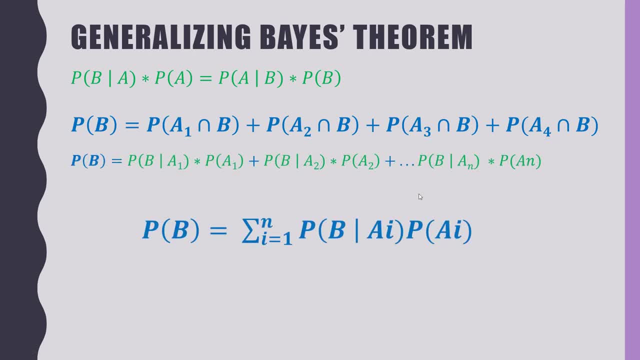 take a moment to look at it. so, that being said, we've now used our famous sigma notation here and looking here, what i've done is i've changed this to go from one to two to three, to four, to one to two, all the way up to subscript n, in other words, the probability of b occurring. 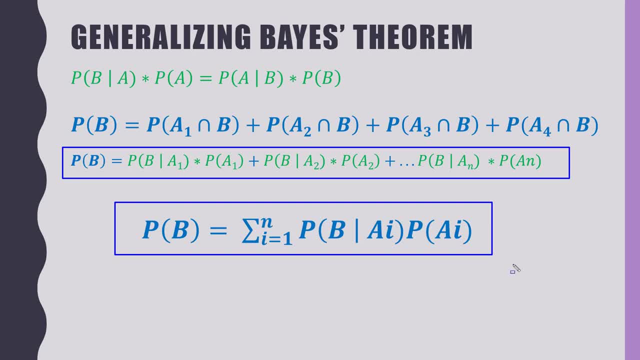 is that. do you agree with that? obviously, i could also do the same thing with the probability of a right agreed. so if we were looking at events where i want to know the probability of a, i could also do the same thing with the probability of a. then, of course, this would be an a, this would be an a, this would be b, i and this. 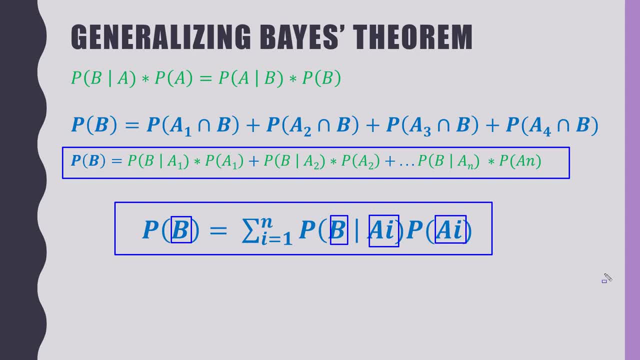 would be b, i right. so you understand that's the same idea. we feel okay about that sum formula there. okay, that is total probability of b. that's what that concept is. total is called total probability. so let's look at what's. i'm going to surprise myself. i don't remember what the next 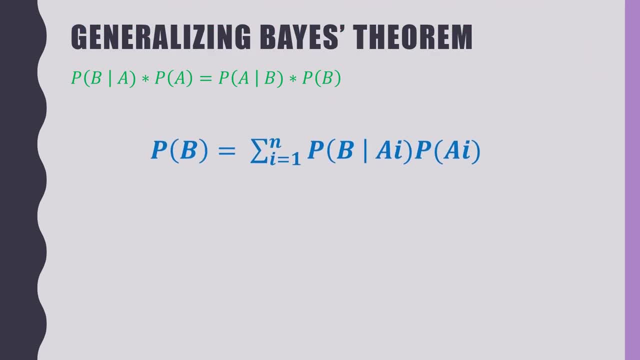 slide is, but it's going to be fun, i promise. all right, let's just be moving stuff out of the way, okay, all right. so this is now. this is the total probability. well, what we're going to see in a minute when we look at the probability where 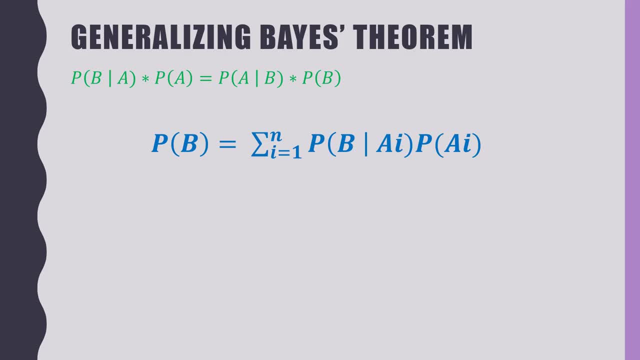 with bay's formula, where the denominator is the probability of b. we're going to plug that in instead, right? because, remember, probability of b given a is equal to the probability of a given b times probability b divided by probability of a right. so we can use this for the denominator. 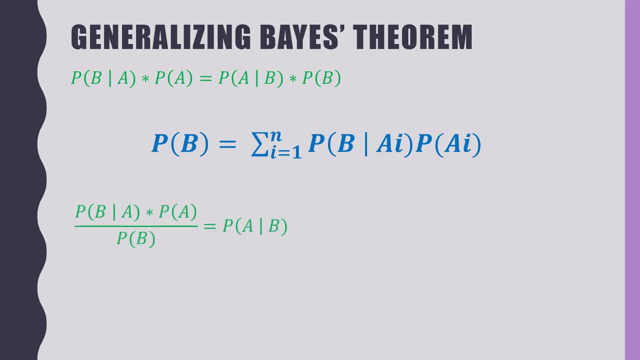 this formula here again. this is one i just sort of recited a second ago and this one: do you agree that these? this is the same idea, right? i just rearranged it, so this is a scenario where we're going to use that to plug in right here. okay, so i'm just re putting the equal the the formula on: 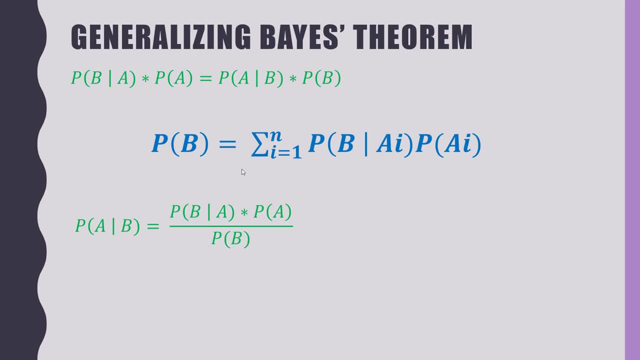 the left, but it's the same thing. all right, since we all understand this formula, we agree with it. we're going to substitute that as a formula and we're going to plug in this formula here, as i mentioned, for the denominator of the original formula there and now. this is the final. 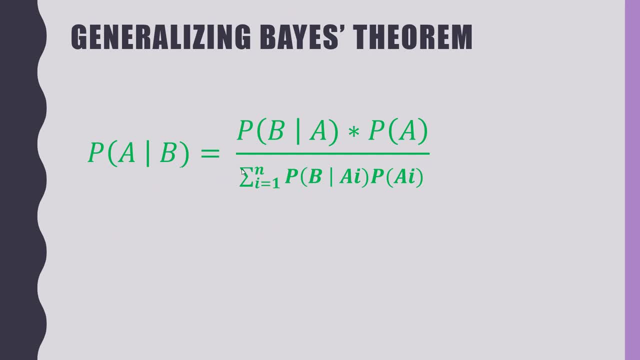 complete base theorem with everything generalized. there's one little thing we need to tweak, which is that adding the subscript for the a's there right. so the probability of a subscript i given that b did occur, is the probability of b given a subscript i which is not subscripted. 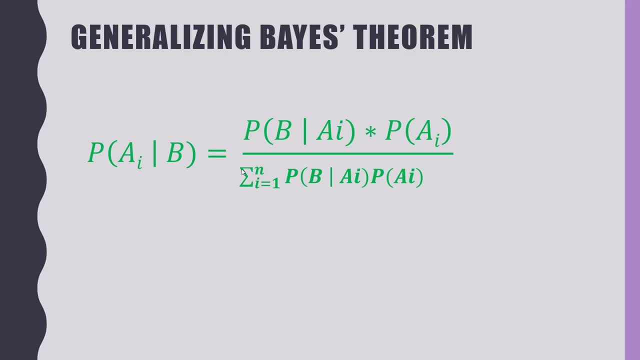 but it should be and i'm not going to fix it- times the probability of b given a subscript i, which is the probability of a given, uh, probability of a divided by that whole mess we just walked through. how do we feel about that? that is the final generalized formula. 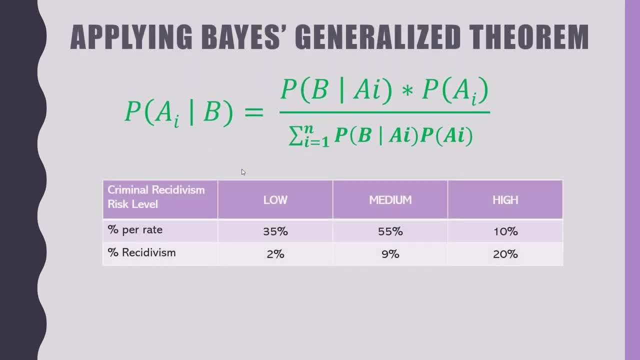 let's take some applications of it. we have here some statistics that are made up. i made these up. i don't know if they're real or not. okay, they're. they're based on some reality. but here's what we're looking at. we have criminals that are ranked. 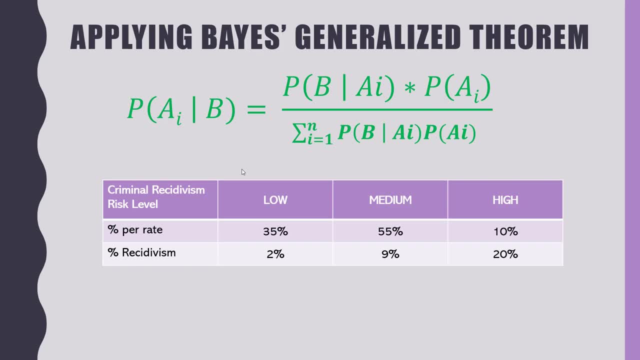 from low risk of recidivism. right, they're going to. they're low chances, they're going to go back to prison. there's a medium chance to go back to prison and there's a high chance they're going to go back to prison. okay, the first row. there is the percentage of low risk criminals: 35 of the. 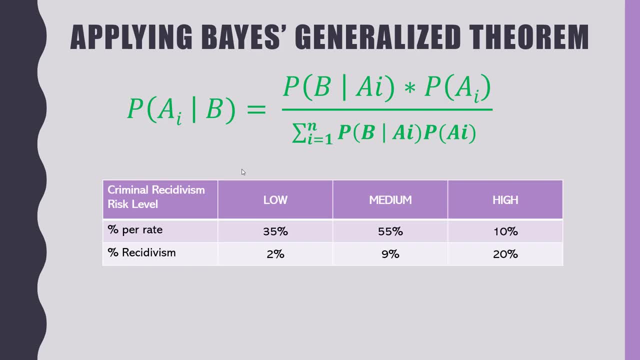 criminals are low risk, 55 are medium risk, 10 are high risk. okay, then the actual percentage of recidivism rate. the low risk criminals have a two percent recidivism rate. okay, so think about that for just a minute. make sure we understand that number. we have 100. 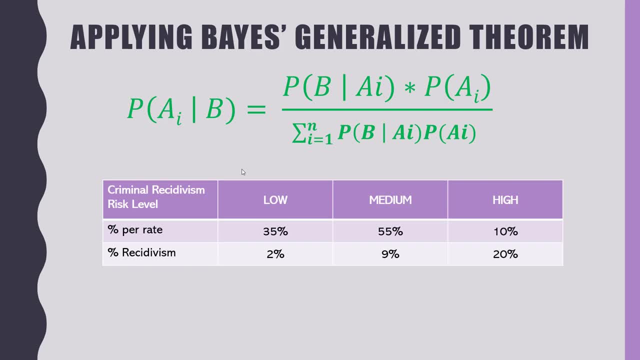 criminals, 35 of them are low risk. of those 35, two percent of them will actually commit crime again. that makes sense because they're low risk, right, medium risk criminals. of those 55 percent, nine percent of them will create a commit a crime again. and then of the high risk criminals, which 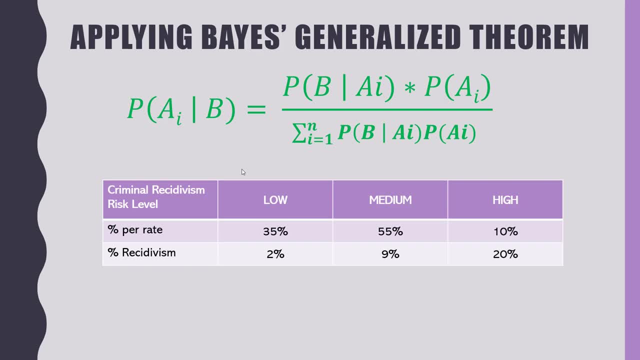 is a very small group. there's only 10 percent of the criminal population are high risk and then low risk, but 20 of those 10 will will repeat offend. okay, so we do. we understand the numbers, though. and now if i were to ask you something like: oh that, what's the probability that any 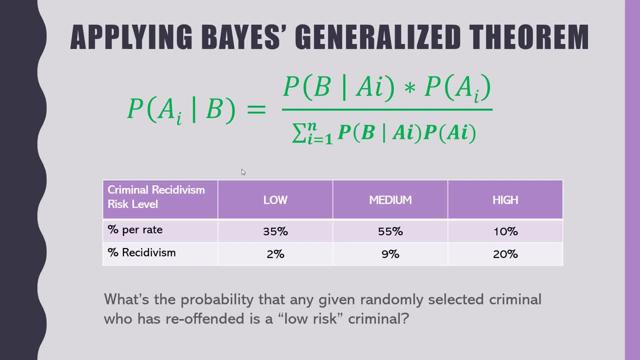 given randomly selected criminal, so the entire criminal population is: randomly grab one, and what's the probability? and? and he has re-offended. so i grab a random criminal who has re-offended, what's the probability that that criminal is low risk? that seems like a hard question to answer, doesn't it? 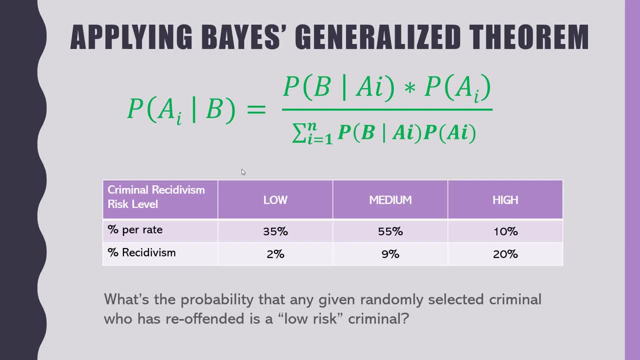 we can, we, we can. we can answer it now with the with base formula. okay, we can plug this in, so let's look at how this would all apply. so here's our formula again. i just moved it down so we can look at it. let's just let's. 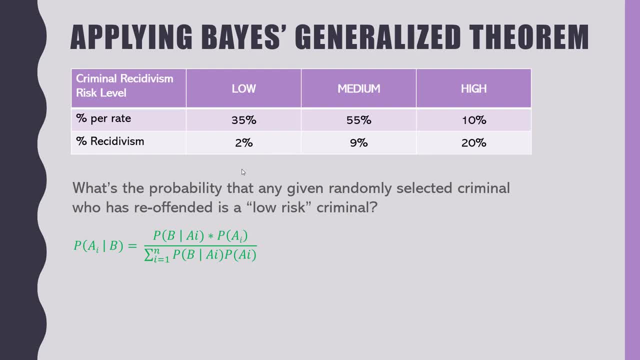 plug in what we know. what's the probability of b given a? and again, that should be subscripted. i'm not going to change it, i'm just going to keep reminding us that it should be a subscript. i must have missed it when i was making that slide. what is the probability of b given a? 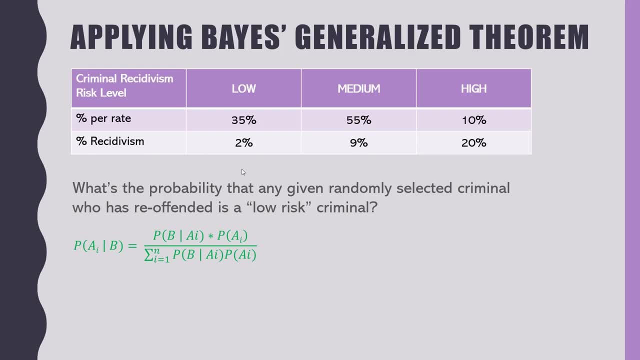 well, what is it? what's the probability of a, what is b and what is a in this scenario? so the thing that we know is that they are a reoffender. that's the given right. so we want to know the probability that they're low risk, given that they're reoffender. so a is our low risk, b is the. 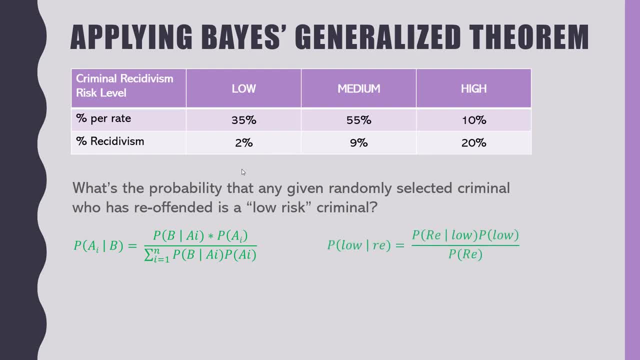 reoffender, right? does that make sense? so if we just- i think i've changed it, yeah, i changed it to look like that, okay, so we're asking: what's the probability that you're low risk, given that you are a reoffender? that is equal to the probability of being a reoffender, given that you are low risk. 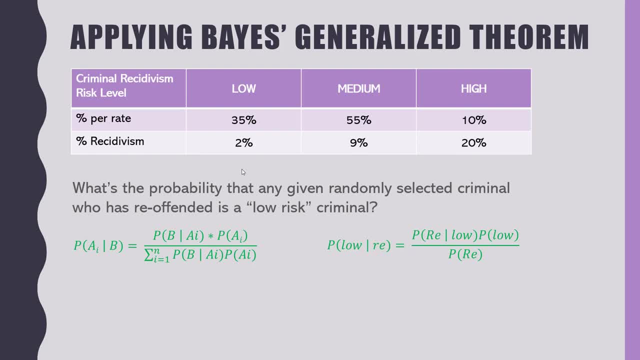 times the probability of you being a low risk divided by the probability of you being a reoffender. now look at the, the numerator there. that's pretty easy. i think we can see that those numbers pretty simply: what's the probability of being a reoffender given that you are a low risk? 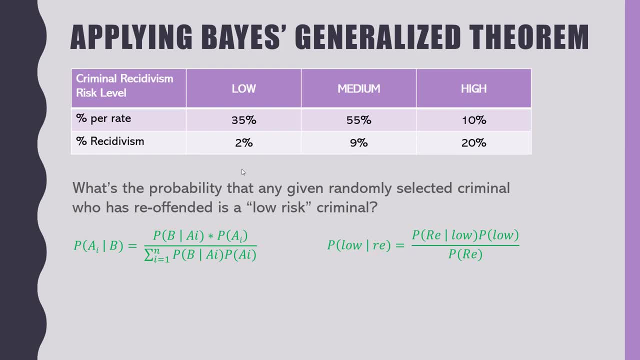 that number is given to us. what is it? two percent, right? the probability of being a reoffender, given that you have that, you are a low risk- is two percent. that is exactly what these numbers mean here. these numbers mean what's the probability of that given, whatever one of those you are. that's what those numbers are right. 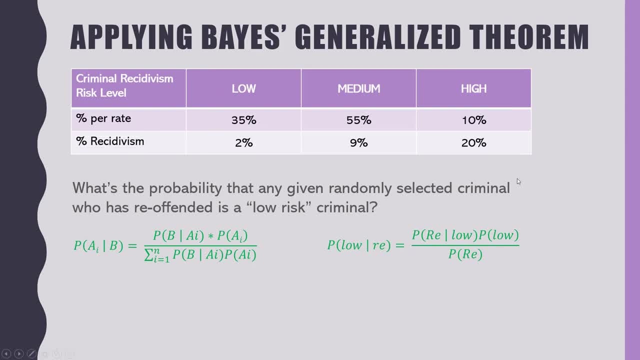 so that's easy enough. what is the probability that you are a low risk criminal? 35, so the top is easy. right, it's two percent times 35, right, that's pretty easy, okay, probability of being a repeat offender: that's a little trickier. well, knowing what we know about the total, 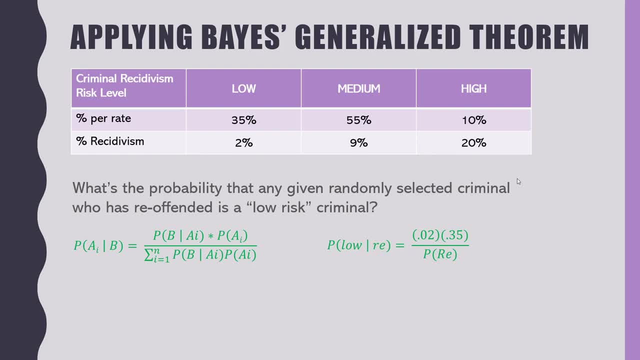 probability that we've been spending the last few minutes on, in that that, with our sigma notation over there, how can we answer this? wouldn't it mean what we did for the numerator, except for the rest of them as well? exactly right, yeah, so it's the probability. so we got these two numbers. very good, we got these two numbers here. 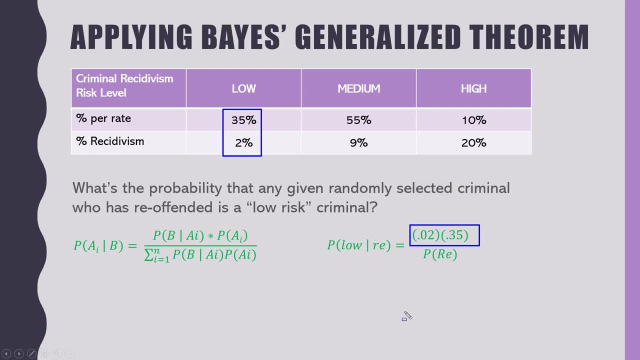 by multiplying these two numbers. right, and we do, and do we understand why that is? because that is the probability of b given a times the probability of a right. well, we want to know that, the sum of all of those. so we want to know the sum of that. 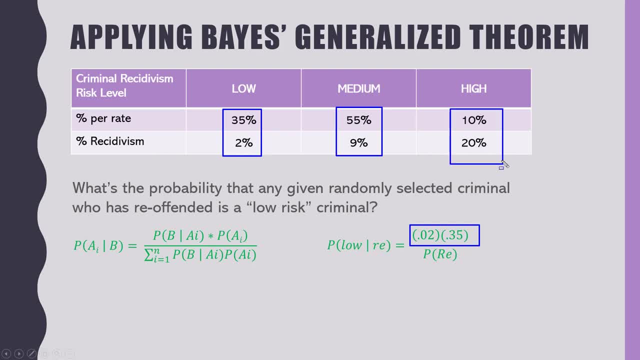 plus the sum, plus that, plus that, that will be our denominator. that make sense. so we have that for our denominator. do you agree with that? do you understand it? whether you agree with it or not, it is true. so the real question is: do you understand it, right? yeah, so now let's do a little bit of math. 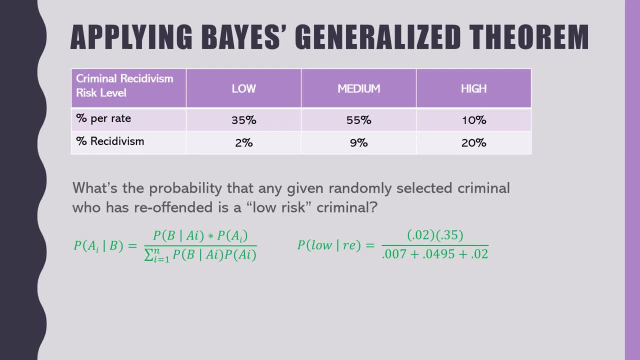 here and let's just kind of shrink this stuff up a little bit. we get those numbers on the bottom. i just did the math for you. if you want to plug them in your calculator, verify them- right, you can, and then let's, let's combine them a little bit more and we get. ultimately, we're going to have this divided by that. 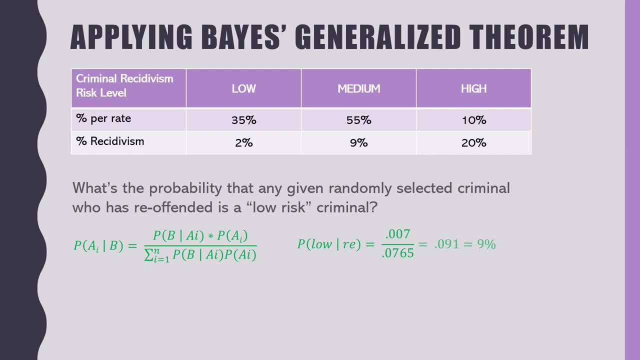 0.007 divided by 0.0765, which ultimately gives us a nine percent chance that we are a low risk criminal if we've re-offended. so when we look at the fact that that 35 of the criminals are low risk and but their recidivism rate is low, and so this, this, this disproportion here, is what makes that, 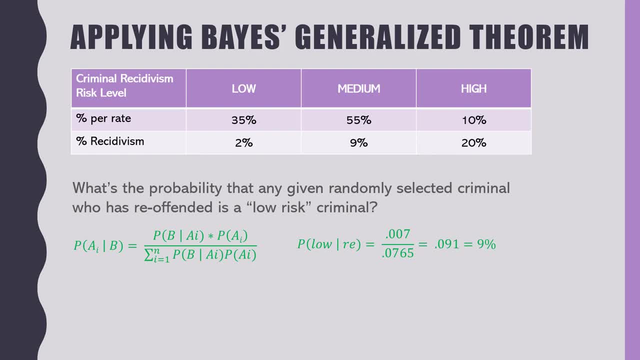 number go a lot lower than we might have thought. if we were to do the same thing for a high risk person, we'd see a lot higher risk than we might have thought. if we were to do the same thing for a high risk person, we'd see a lot higher. 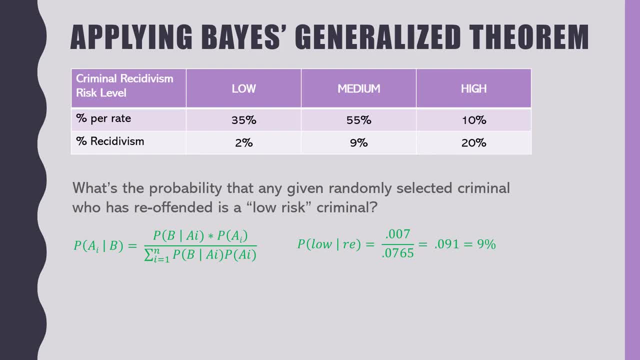 numbers here, but they won't necessarily be what we might have thought. now, how many of you, and maybe you? the answer is yes, but that's okay if you did see this, if you didn't see it, it's also okay. but how many of you thought: well, obviously it's going to be around 10 percent, or did some of you? 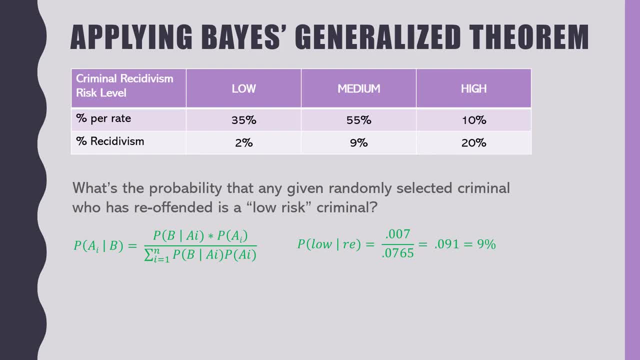 think it's going to be higher. some of you think is going to be a lot lower. anybody want to throw that out real quick. any thoughts on that? i thought it was going to be lower, lower, okay, like how, like one percent or something like that. or like five, okay, about half. so yeah. 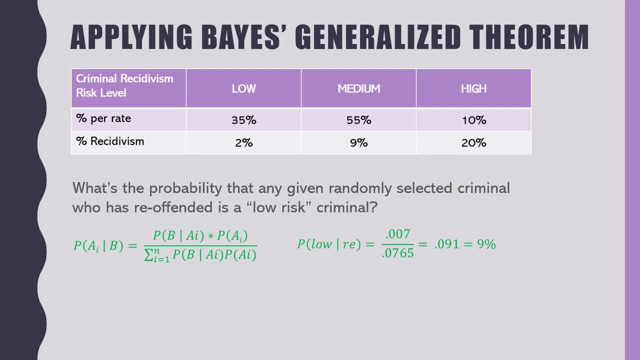 and i don't mean this like negatively, but that's way different than what it actually is, right, it's, it's way off, and so a lot of times our intuitive thinking is off until we actually apply the numbers, and so that's why this formula is so important- is that it helps us see things. 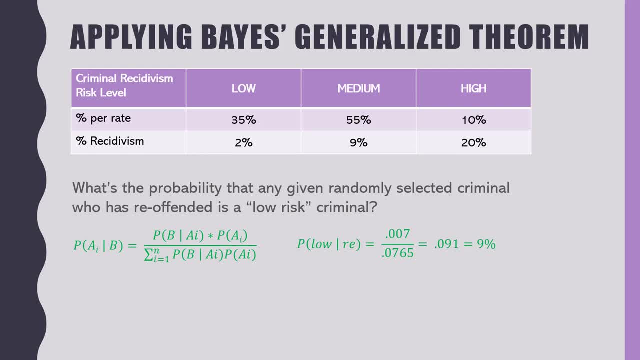 that are right there that we didn't recognize and we're going to see that when we get into this other question we asked about earlier now. so again, the question was: what's the probability that any given randomly selected criminal who has reoffended is low risk? 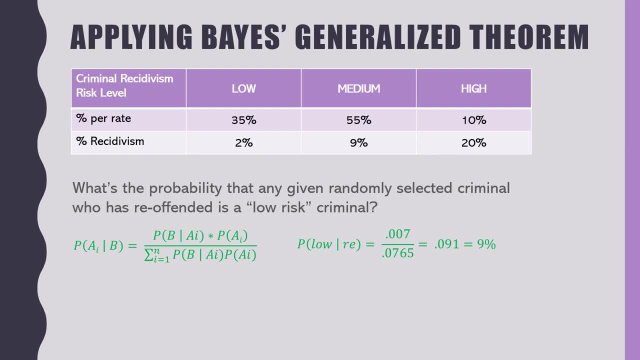 and it seems like it would be pretty darn low. and nine percent is higher than i would have thought too. okay, okay, very good, taking percentages of percentages. yes, i know, when i first asked the question i noticed you just threw out some numbers right off the bat. where did those come from? i'm 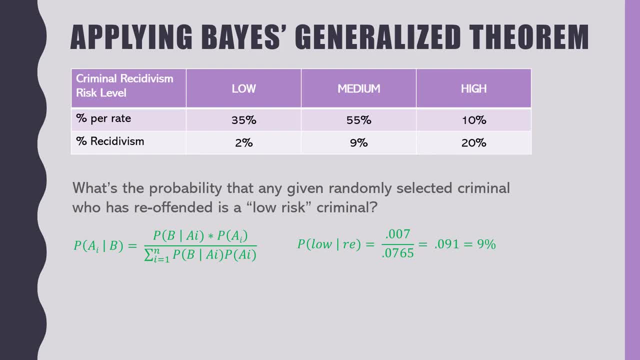 curious. oh, it was the multiplication of like the two over 36, because i really had to take it for time so i just kind of guessed it was somewhere on there. oh, what does that all end up being? is that close like two divided by 36? where are you getting the 36 from? 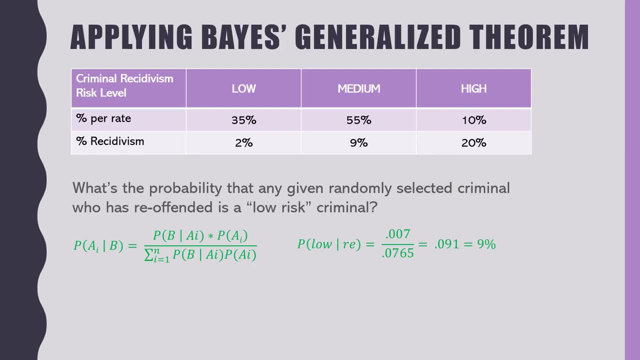 oh, i was just adding up some percentage. it wasn't completely, it was just kind of a guess. okay, well, i'm curious of what that ends up being. it's like five percent, five percent. yeah, the reason i want you to calculate that is because it's just more evidence that oftentimes we look at the facts and our our natural brain. 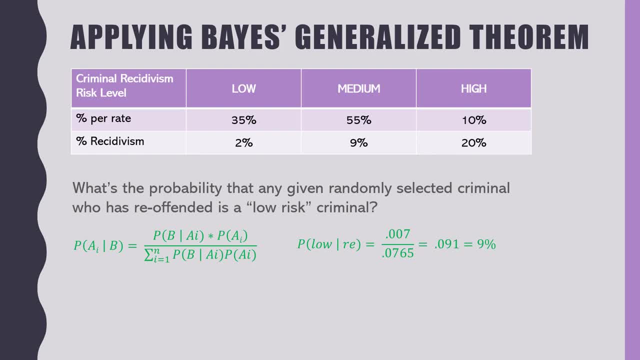 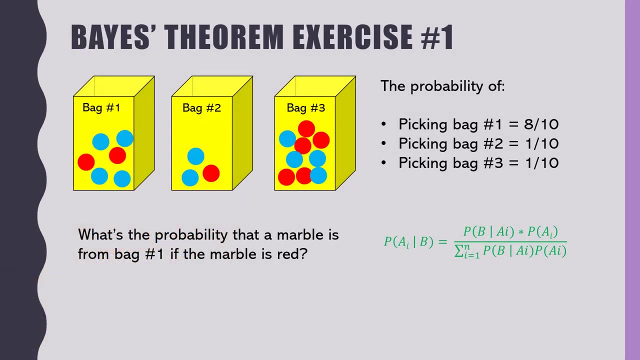 thinks: oh yeah, it's about this, and sometimes we're way off. we were off by about half, right, so this is that's why this formula is so important. okay, good, i'm glad that that we did that little experiment there. okay, do the whiteboards? uh, looking around the room, it looks like we all got it correct. let's just make sure. real briefly, 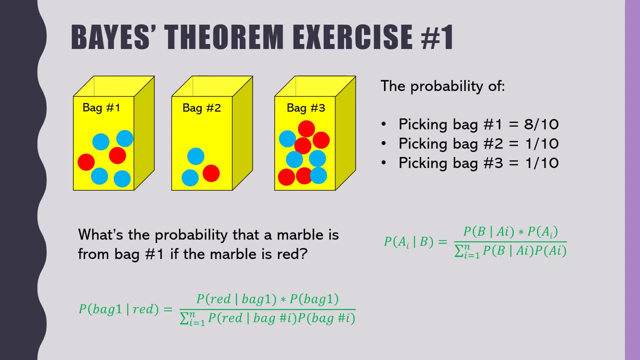 this is the question that's being asked here, and it's always good to form the question in terms of variables that make a little bit more sense. so i'm asking: what's the probability that the marble came from baguette one, given that it was red? That is the question that's being asked, And if you substitute the 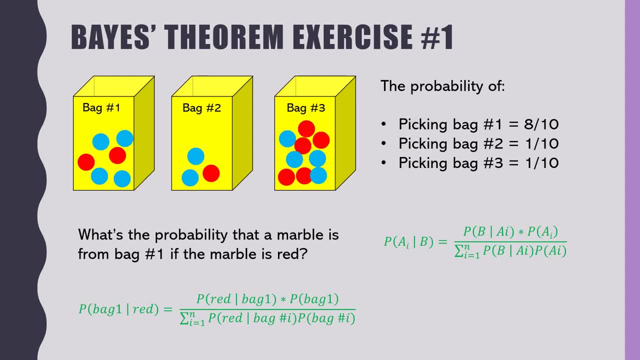 words bag one and red. throughout the formula, you'll get that little green thing on the bottom there, right, We can plug in the top numbers. That's pretty easy, because we know the probability of it being red, which was two out of six, given that it came from bag one, which is two out of. 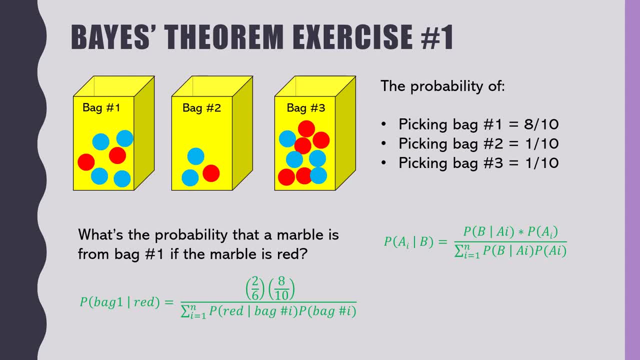 six, right, We can see that by looking at the picture And we know the probability of picking bag one, which is eight out of ten. That's pretty easy. The bottom one. we have to sum everything up right, Just like we did before. So I have to multiply, whatever the probability is here. 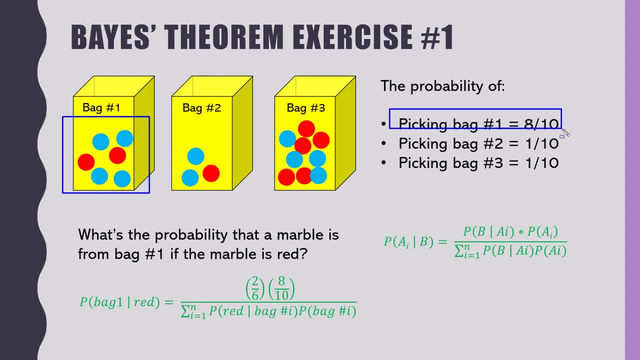 which is two out of six times eight-tenths right Plus one-third times one-tenth right Plus, if I remember right, that's five out of nine. There's five reds and a total of nine marbles times one-third. 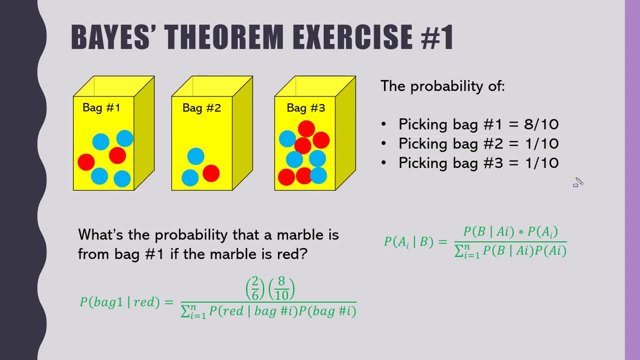 So you multiply and add all that together and that will be your denominator, right? And so I think I just plugged in those numbers for you, like that. Everybody understand that, Hopefully, I think you do, because you all got it correct And I'm just going to walk through the math. real, 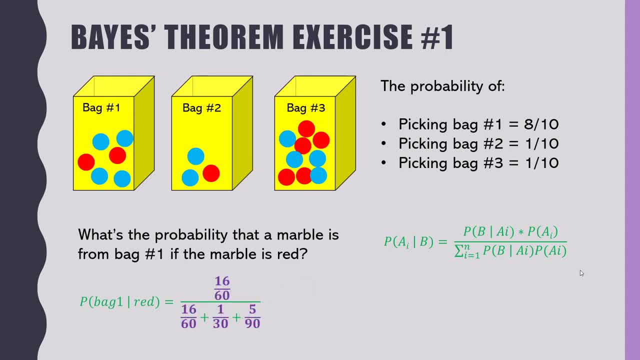 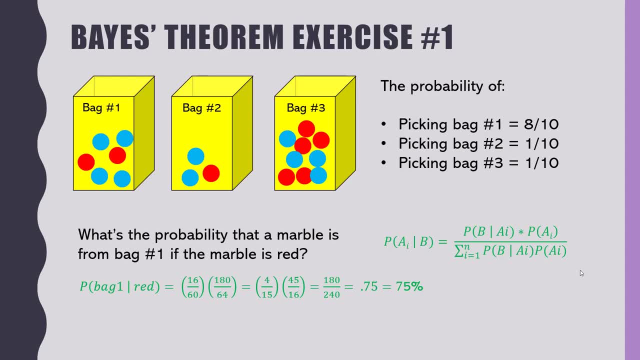 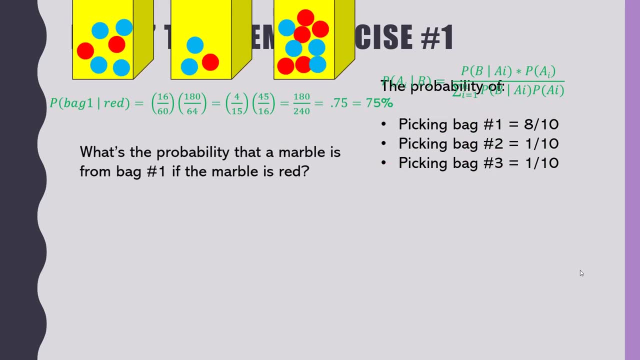 all over the board. So you guys got it correct. So we understand that. I think we're good there. Let's look at another way, though, that we can figure out the denominator right. This is a probability tree, So I moved the bags out of the way, the pictures, and I just put on the right. 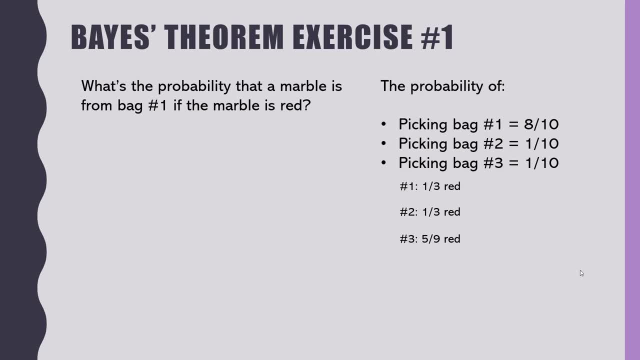 there the probability of one is for the actual reds is one-third of red, one-third of red and five-ninth of red. okay, So we have a starting point And we're a probability tree. It's a binary decision tree Sometimes. Sometimes it's trinary, which is kind of going to be right now. 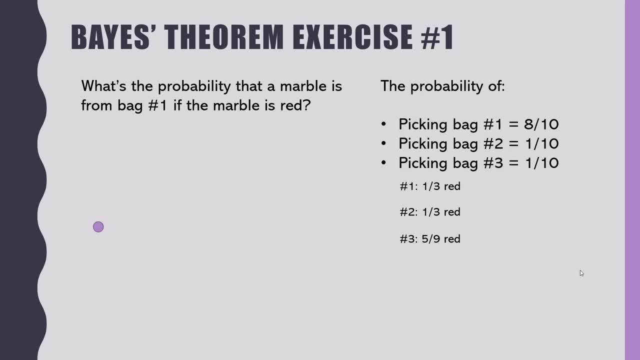 right. So what's going to happen here? We've got three choices, with our starting point: picking a bag- right. So three branches. I could pick bag one, pick bag two or pick bag three From bag one. it is binary, It's red or blue, That's it. And, by the way, we know that there's. 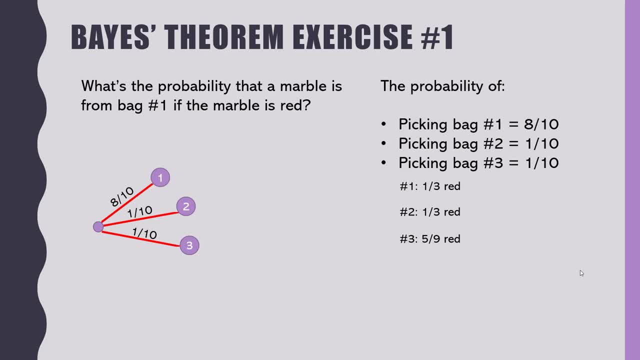 an eight-tenths percent chance I'm going to take, or an eight-tenths chance I'm going to get, one, and so forth. I just plugged in those numbers there, right? Okay, Now, once I'm in the bag, 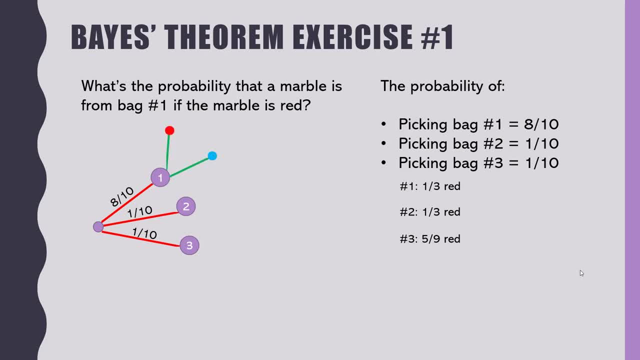 bag one, bag two or bag three. I will make a decision to either pick the red one or the blue one. And I say: make a decision. but we're all. this is all blind, right? We don't? I'm not looking. 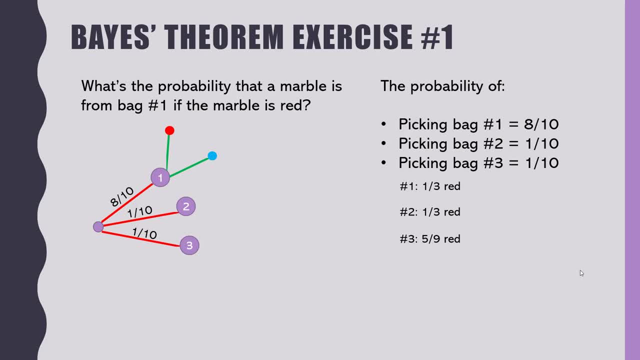 in there, Because if the probability of me getting a red when I'm looking and I can see what ball I'm going to pick, well it's going to be 100% because I'm going to pick a red one, right? So that's not. 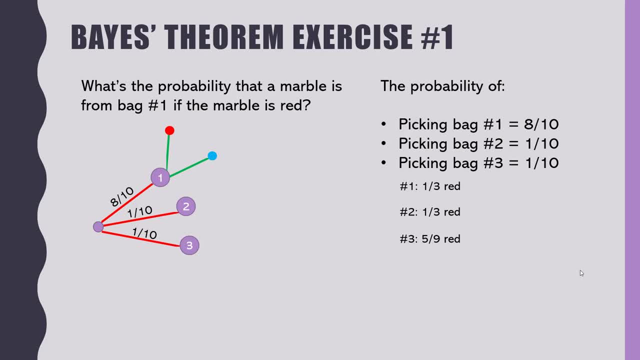 what we're asking. We're just saying if you're blindfolded and you reached in and just randomly grabbed one, okay, So what's the probability from bag one that it's going to be red? We know that number and it's on the right there and we'll look at it in just a moment. 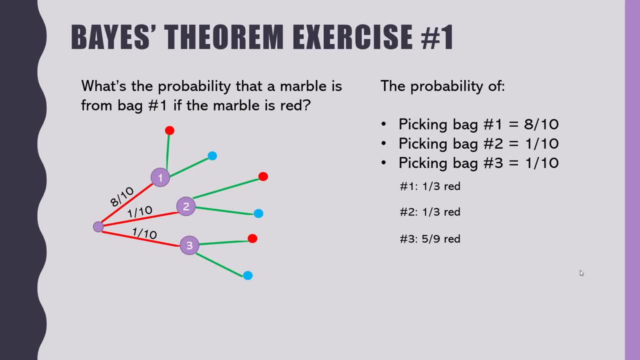 But as you can see from bag two and bag three, again, we'll either pick red or we'll pick blue. So this little binary tree- not binary- this decision tree, can help us make a decision of what the what's that? It's a weighted graph, yeah, All right, So now. and it's also a tree. 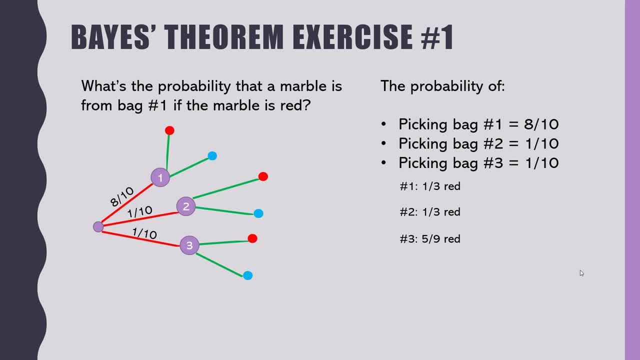 because there's a root and there's no loops right, And a tree is a graph. Okay, So now we can put those values where they are. So now we can put those values where they are. So now we can put those values where they belong right. One-third of the time you'll get a red in bag one. 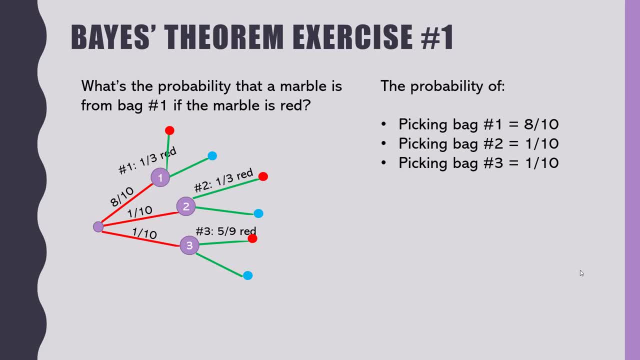 also in bag two, and then, five-ninths of the time, you'll get a red in bag three. right, I'm just going to clean that up a little bit there. And then, if that's the case, if one-third of the time, 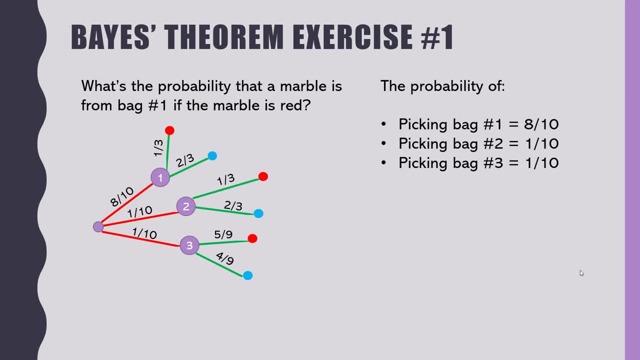 you get red, that means two-thirds of the time you'll get blue right. We agree with all the numbers on the graph. So you can draw this kind of a picture to help you get the total probability for your denominator when you're doing a Bayes calculation. Now what we're looking for. 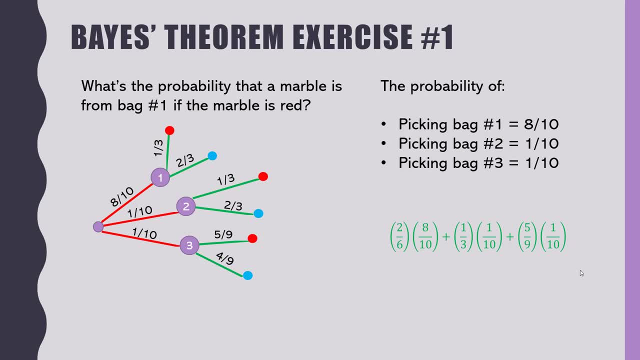 again, it's the path to red. We're going to add up all the paths to red. Well, what are the paths to red? Well, there's the first path, that goes eight-tenths to one-third right, Or two-sixths. 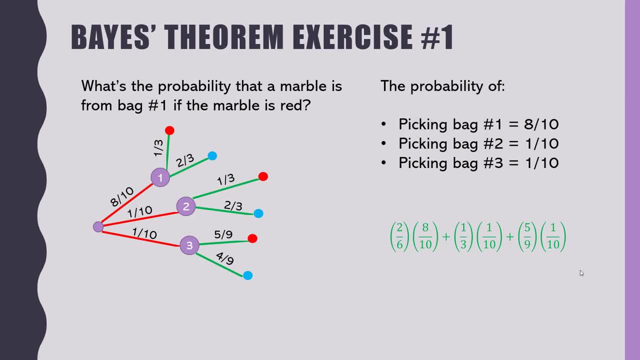 plus the path that goes one-tenth to one-third, plus the path that goes one-tenth to five-ninths. I got those not in the right order there, but you get the idea. You see that To the whiteboards. 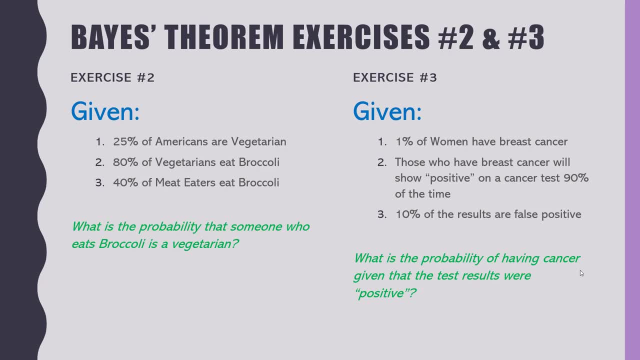 Looking around the room, I think you guys got everything correct, So here we go. Let's look at the one on the left here. Notice what I did. I substituted out variables that seemed to fit a little easier. Rather than trying to say A equals this and B equals that, I said V for vegetarian. 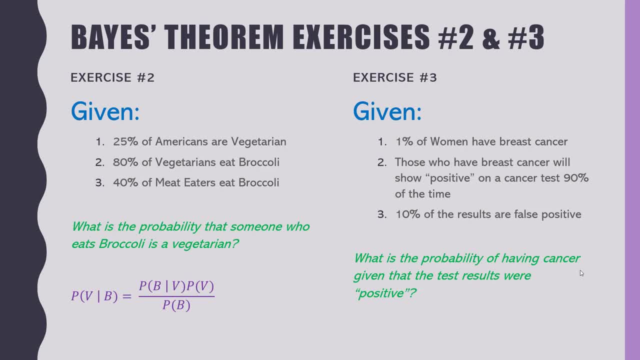 B for broccoli eater right. So the probability of being a vegetarian, given that you eat broccoli, is the probability of eating broccoli given that you're vegetarian times: the probability of being a vegetarian divided by the probability of eating broccoli. So that's the probability of being a. 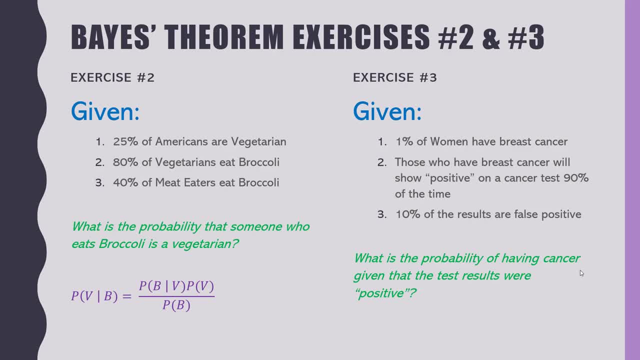 vegetarian divided by the total probability of being a broccoli eater. right, We all agree with the equation. We can do now some plug and play here and substitute the top two numbers. Those are always easy to get right. What's the probability of being a broccoli eater? 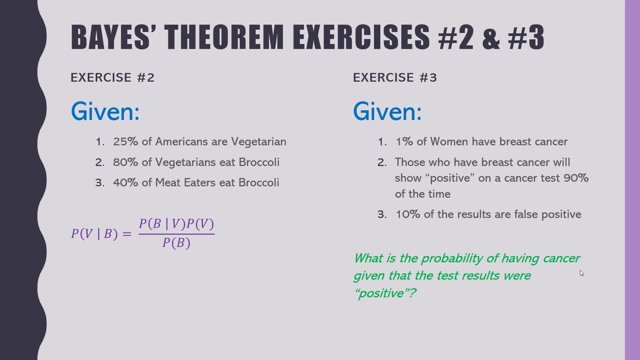 given that you're a vegetarian. That's bullet point number two. right, Probability of being a vegetarian, bullet point number one. So the givens are there Now. what's the probability of being a broccoli eater? What's the probability of being a vegetarian? What's the probability of? 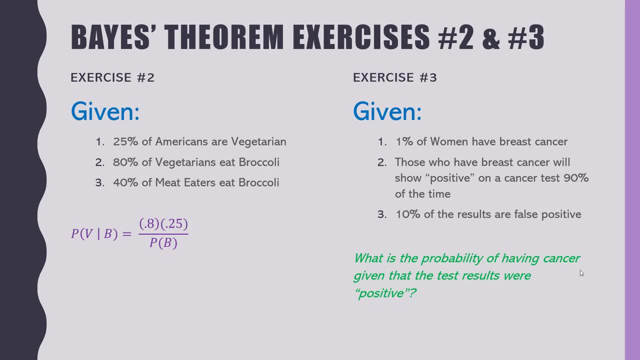 being a broccoli eater. Well, there's two kinds of broccoli eaters: There's vegetarians and there's non-vegetarians, right, Okay? So how do we figure this out? Well, we're going to use a tree for this, And this is a simple tree, And remember, the trees always start wherever your starting. 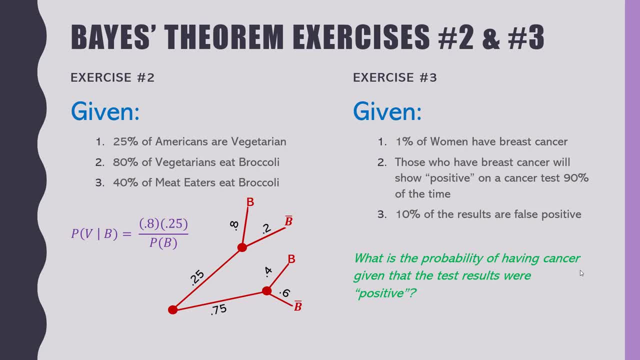 point is you're going to make whatever possible decisions there are And then, once you arrived at that place, you can make whatever possible decisions are next. So in this case, we started off with this starting point here And we decided to make the decision being that there are vegetarians- 25%, which I'm not sure how. 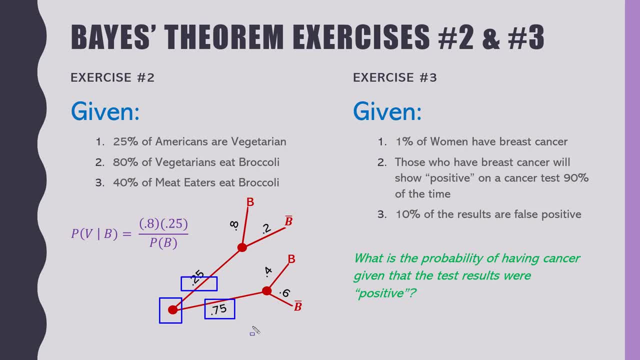 to get around that box there. Sorry about that. And then 75% are not vegetarians. right, You have one or the other. Once you get there, then 80% of these vegetarians here eat broccoli and 20% don't. 40% of the non-vegetarians eat broccoli and 60% don't. That's it What we're. 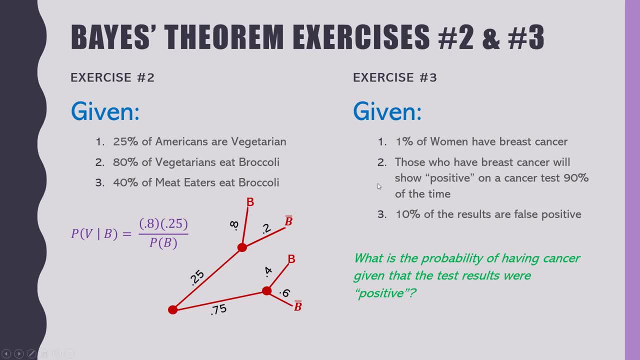 going to do is we're going to multiply the total probability of being a broccoli eater, okay? Well, we just look at the paths. There's the blue path, right there, right, And then there is the green path. We add those two paths together. First, we multiply the numbers along the way, so 0.25 times. 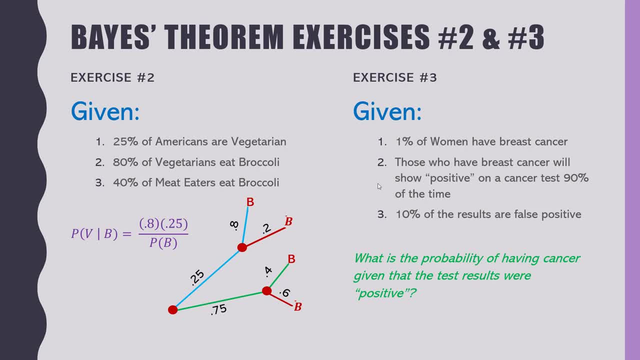 0.8 plus 0.75 times 0.4, right, We get this formula right here. That's our total probability, okay, Which is 0.5.. And then we multiply that by 0.5, and we get the total probability of being a vegetarian. 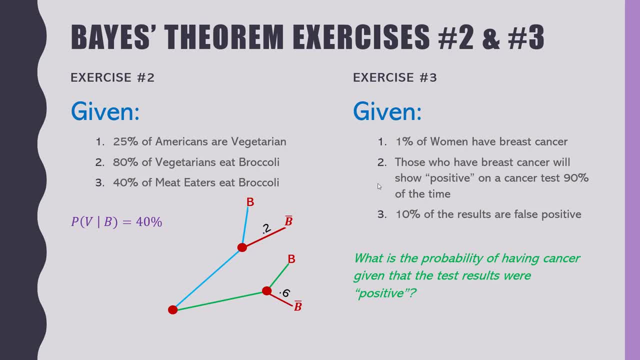 given that you eat broccoli, is 40% Questions about that Pretty straightforward, I think It's mostly plug and play. It's just about recognizing what data do I actually know and what can I figure out? Because I can figure out what the total probability of whatever my 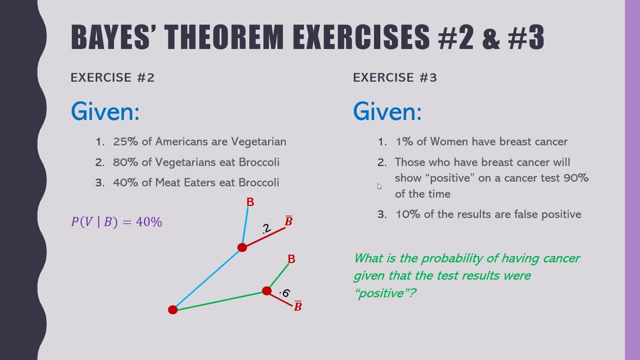 denominator is with what was given to me. All right, let's take a look at the next one. So that's just putting the question back for us. Let's look at the exercise number three Again. notice what I did here. I put in a plus sign for positive and C for cancer, right, Just? 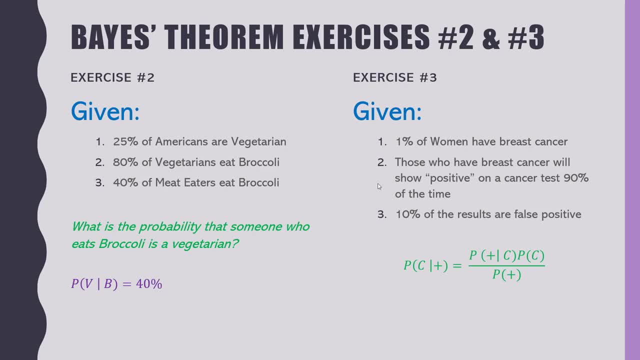 to make it easy to write down: What's the probability that I have cancer, given that I had a positive result test result? Well, it's the probability that it's positive, given that I have cancer, times the probability of having cancer divided by the probability of. 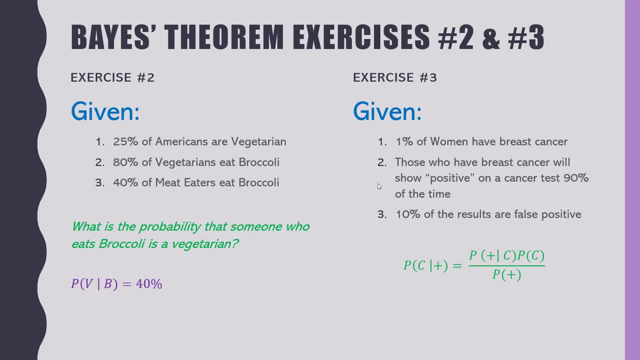 getting a positive, which will be the total probability of all ways to get positive, Because there are multiple ways to get a positive right: Getting a positive when you do have cancer, along with getting a positive when you don't have cancer. That's the total probability of. 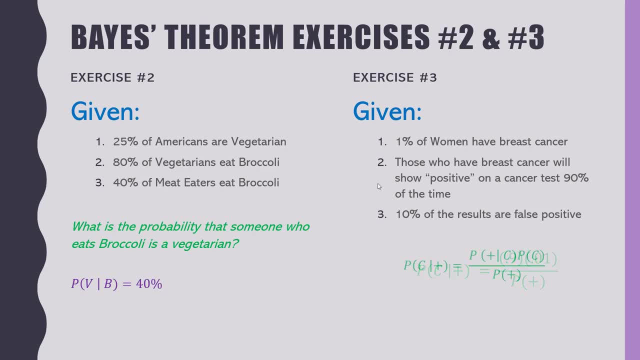 getting a positive. So again, the top numbers are easy right: Probability of getting positive. given that I have cancer, Where is that on my screen here? What bullet point is that 90% right? It's bullet point number two. What's the probability of having cancer? 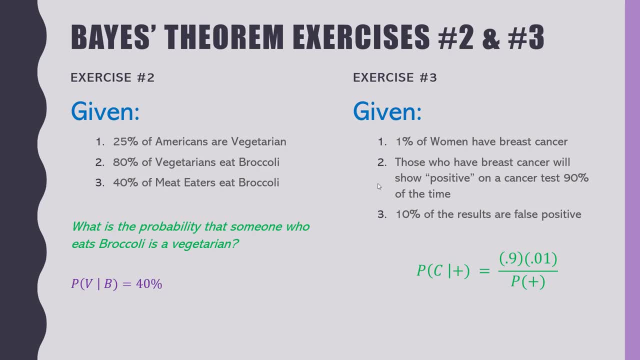 1%. So those are easy to find. What's the probability of having cancer Having a positive result? Well, again, it's the probability of those who don't have cancer getting a positive, plus the probability of those who do have cancer getting a positive. 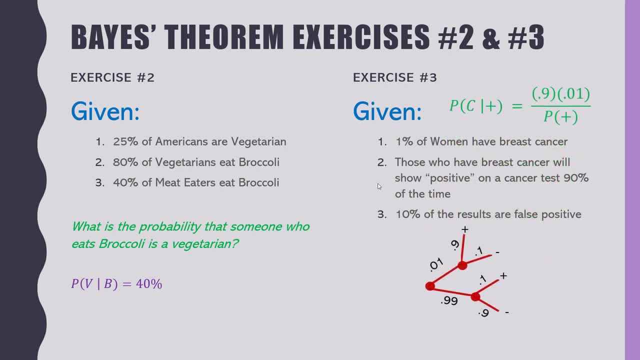 And all the data is there in our bullet points. By the way, these are real numbers as of a couple years ago for women between the ages of 40 and 50, who have for breast cancer statistics. I actually got these numbers from another video about Bayes'. 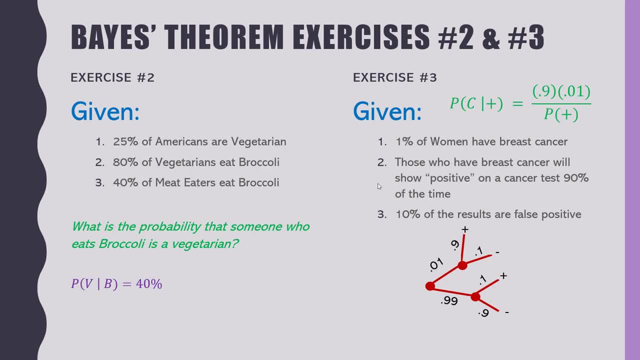 theorem. I just like the example, so I'm using this. I don't remember the exact video I got it from, but it was it was. the numbers are correct. Okay, so take a look at our path again. The far left, little red dot there. 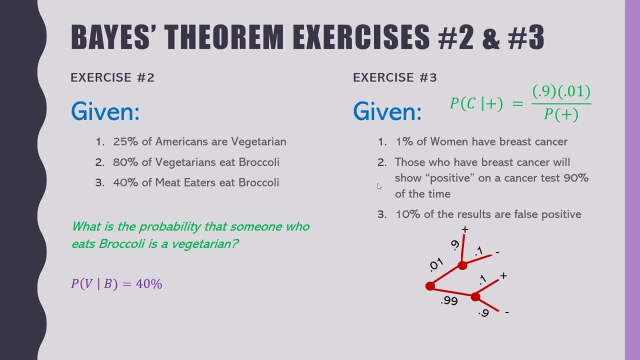 is our starting point, and we had two options. One option is you have cancer. one option is you don't. Option is you don't Once you. so here we have starting point. This means you had cancer. this means you don't. There's a 1% chance that this will happen and a 99% chance that this 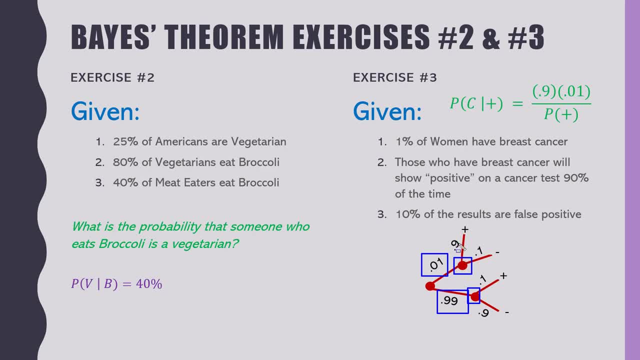 will happen. Once we know that you don't have cancer, we also, or that you do have cancer, we know 90% of the time the test results will be positive and 1% of the and 10% of the time they. 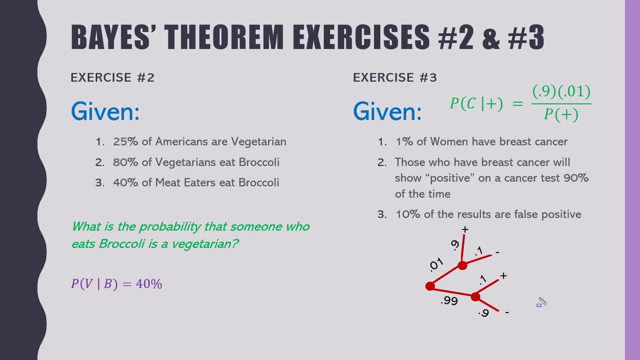 will not. We also know that once we know you don't have cancer, we know that 10% of the time you will get a false positive and 90% of the time it will read negative. Now we have the tree and we know. 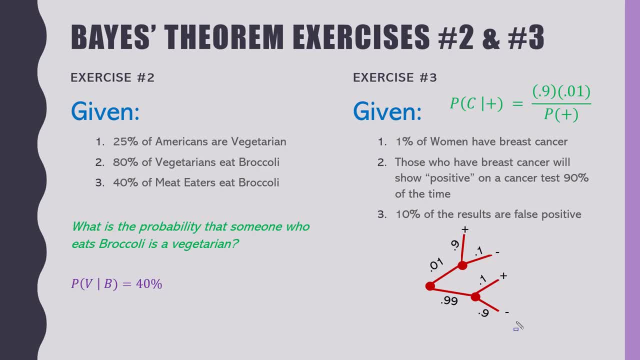 the paths to the each of the different ways to get to a positive result on a cancer test. We can see the first path there in green plus the path there in blue, if you add up 0.01 times 0.9, plus 0.99 times 0.1.. Plug that into the bottom of our formula. 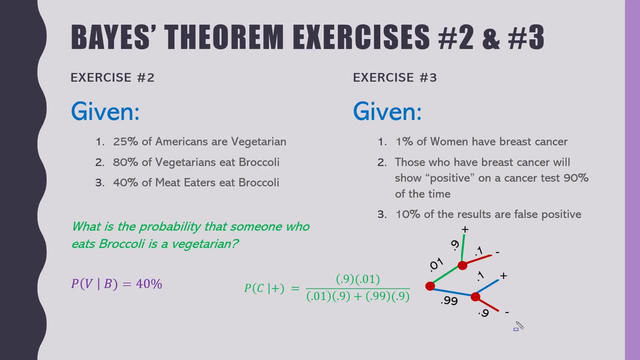 there and you will get those numbers right there. Agreed, When all is said and done, you get 9 over 108, which I believe I saw that fraction on the board a couple times- which is a final answer of 8.3%. So I'm going to put the numbers back up on the screen again. 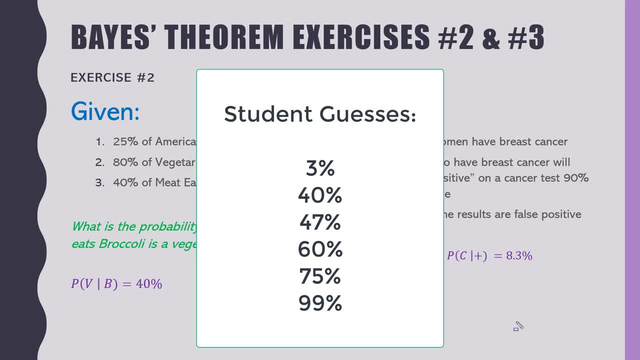 and compare them. The only person who was close. now be honest with me. when you said 3%, were you just being funny or were you genuinely thought it would be that I was just being funny? Okay, so you, yeah. so what did you think? it probably would have been. 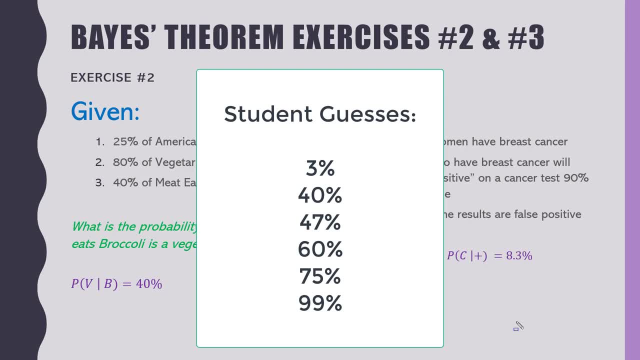 Yeah, okay, good, That's typical. and you see these other numbers here: 40%, 47,, 60,, 75,, 99.. It seems like- and that's just our intuitive brains. well, we say it's intuitive, but it's. 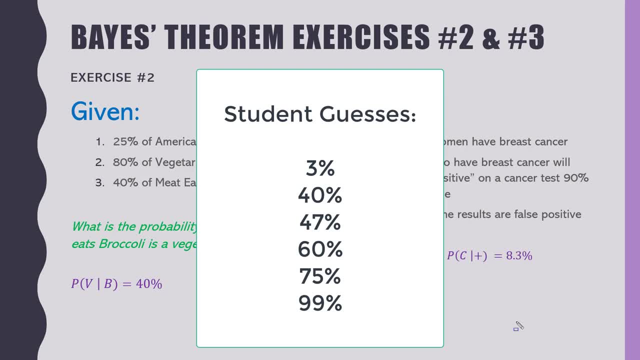 wrong, right. But myself too. you see that and you're like, oh I, 90% of the people who have cancer get a positive hit on a cancer test and I just got a hit on a positive on a cancer test. 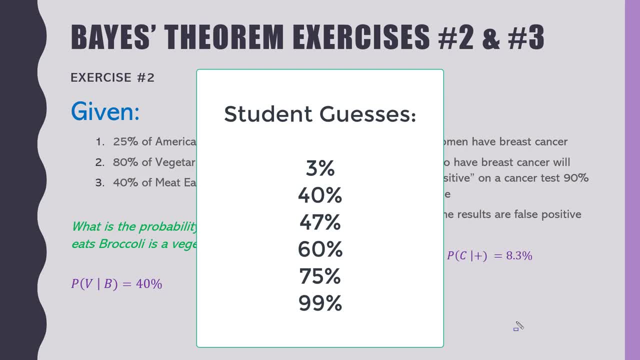 I've probably got cancer right, But it's not even close. There's only an 8% chance that you have cancer if you get positive on a test. It's crazy the difference right? Can they preface that before people get tested? I have no idea. Yeah, I don't know The oncologist. 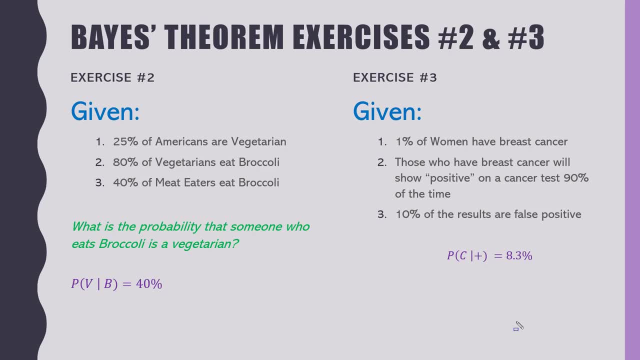 probably, you know, says all right, we need to do another test. That's probably what happens, and so, yeah, I don't know how all that works. I have no idea, but this is a real-world case where Bayes' theorem is useful, because I mean, what if they went from this to all right? 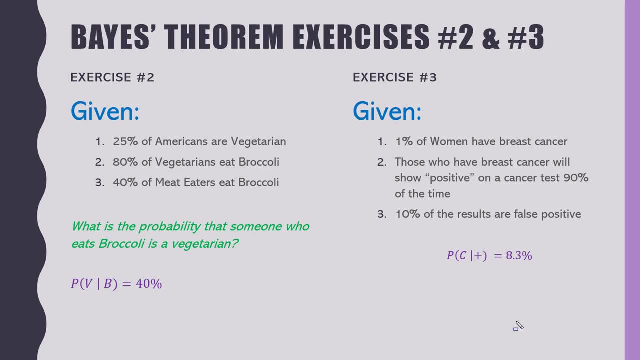 start chemo tomorrow. right, That's nuts. right, There's only an 8% chance you actually have cancer- very slim chance, and what's? I love the fact that you did say 3%, because- and I'm putting- 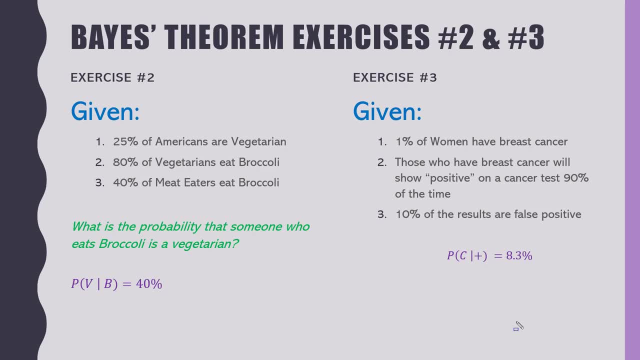 words into your mouth, but essentially your attitude was like: I'm going to say 3, because there's no way it's going to be 3,. right, But then it was closer to 3 than we all thought it might be, but in our minds it seems so ridiculous that it might be that low, which is why you threw. 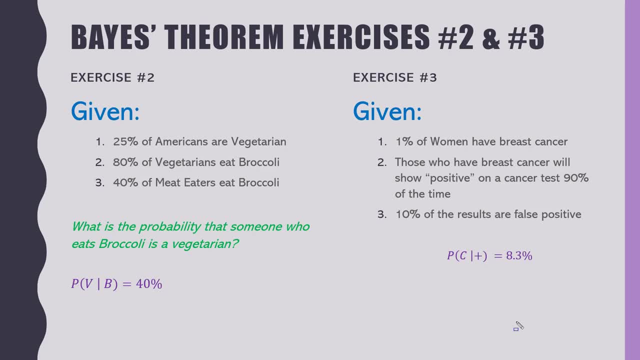 that answer out, I'm assuming. So there we go: 8.3%. So this is this what happens again. we have more data and it helps us update our belief in how accurate something is or whether 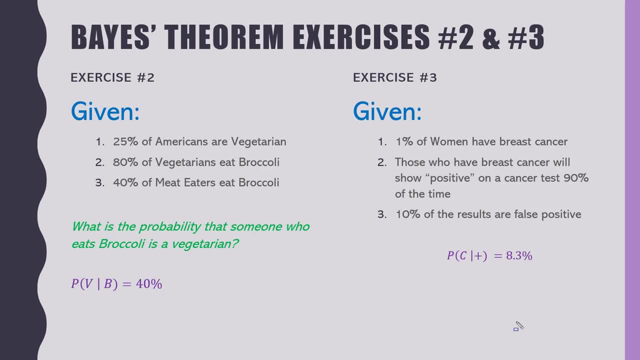 or not, I actually do have cancer and so going in taking the cancer test, the doc says it's positive. My belief is I've got cancer. That's my belief. Once I understand the data and I plug it into the formula, I've updated my 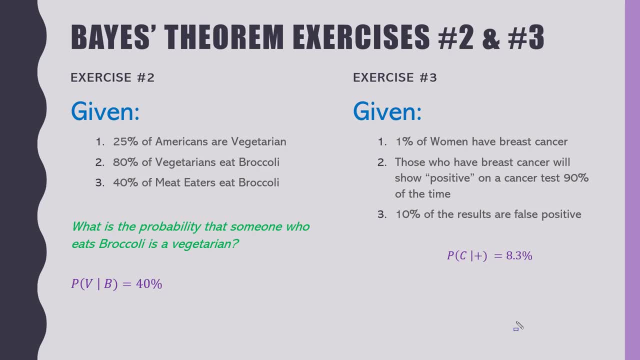 belief. Now I see, yeah, I probably don't have it right. That's how that works Now, using Bayesian thinking in the real world, which we probably won't have time to watch that video, but I will link to. 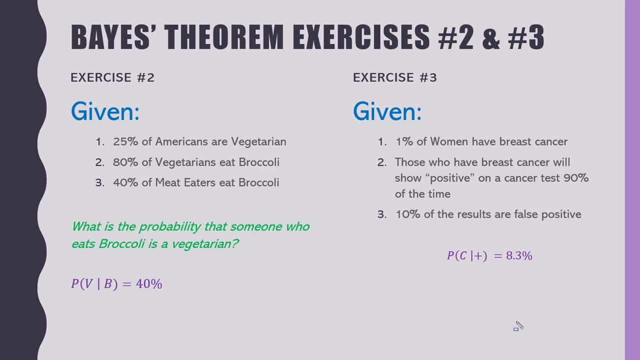 it. you don't just sit there and plug in numbers in your head, but you think through things like this and when you can understand these kind of, you know what is the probability overall of probability of it happening in this little, this little small subset of situations versus this. 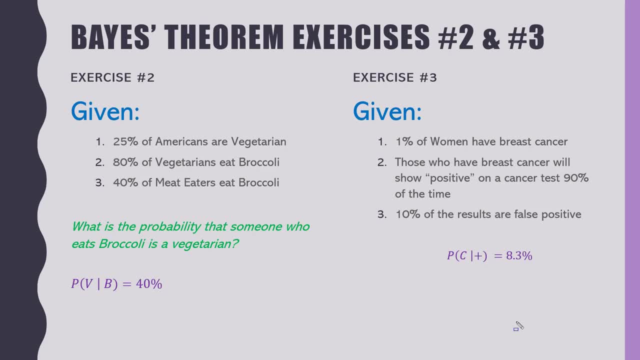 subset of situations and it can change your perspective on things. The more information you have right, the more you know. knowing is half the battle, GI Joe, all that stuff right. We also know like what percent of that cancer test, because not every single person on that. 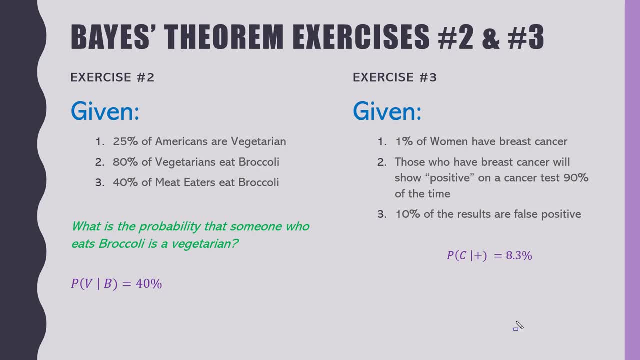 99 would take a cancer test right. So the question is of the people who don't have cancer that take the test. what about all the other people who don't have cancer? What about the people who don't have cancer that didn't take the test? Would knowing that? 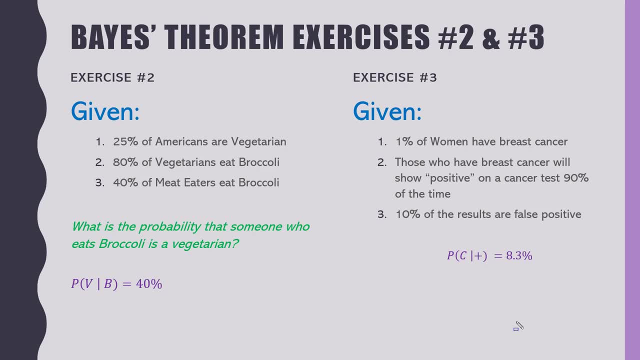 information be useful. So you just assume that everybody takes the test? No, you wouldn't assume that everybody took the test. Let's say right now a million people have taken it. If suddenly 10 million people took it, maybe that number would change The number of. 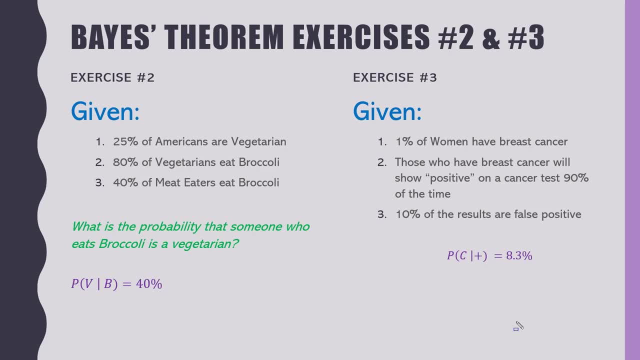 false positives might change. So having a bigger sample set is always useful, for sure. So that's a good point. That probably wouldn't make a difference. Yeah, Yeah, good, But that is. and again, what would we do? We'd update our belief based on the statistics we have. Good question. 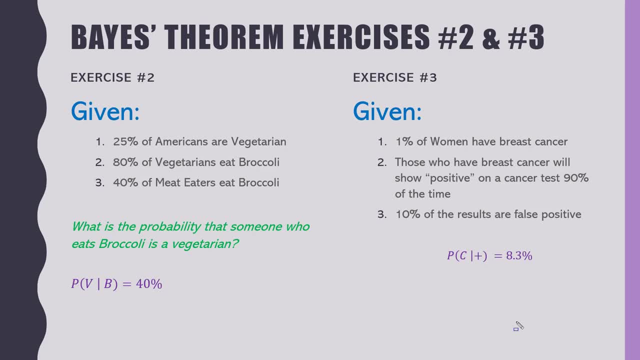 Good questions, But what's the point of all this stuff? Keep an open mind, right? We originally thought all of us, myself included, thought that the answer to this question was going to be at least 50%. None of us thought it was going to be 100%, but we thought it'd be 50,, 60,, 70%, but it 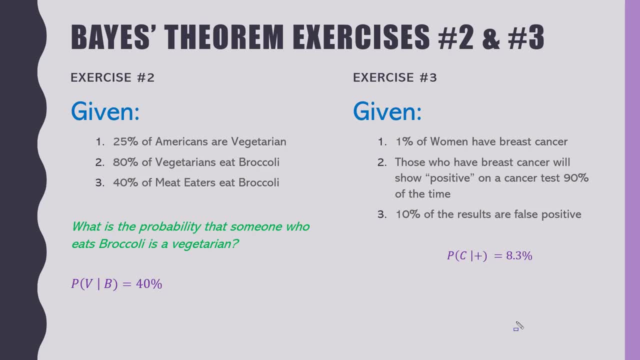 wasn't. So we need to keep an open mind and realize, well, there's more things affecting things than we realize, and this Bayesian thinking can help us update our beliefs based on more and more information. The more information we have, the more we can update our beliefs. So the answer to 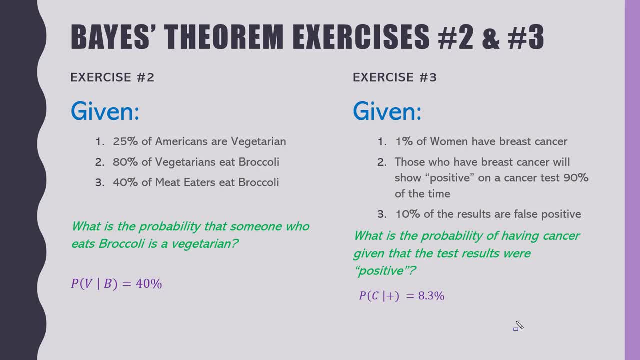 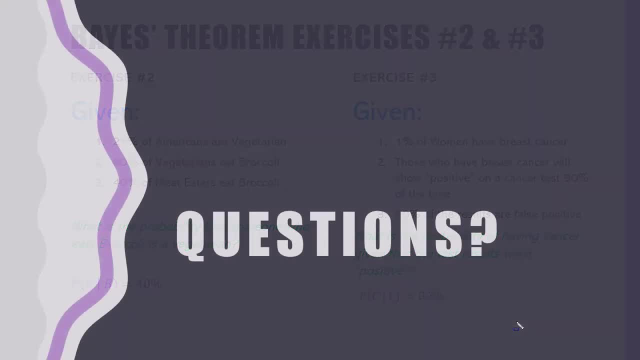 the question: what's the probability of having cancer, given that the test results were positive, is only 8.3%. It's a nice sigh of relief if you did get positive on the test. Any questions about anything that we've talked about today? So just a brief little kind of snapshot here. We're not 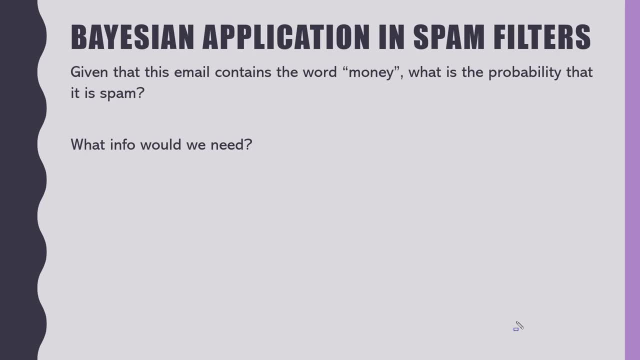 going to do any calculations or anything, but this is the kind of thing that we're- and I've mentioned this a few times before- where Bayesian thinking can be applied, and this is applied in our world as IT people. Given that, this email 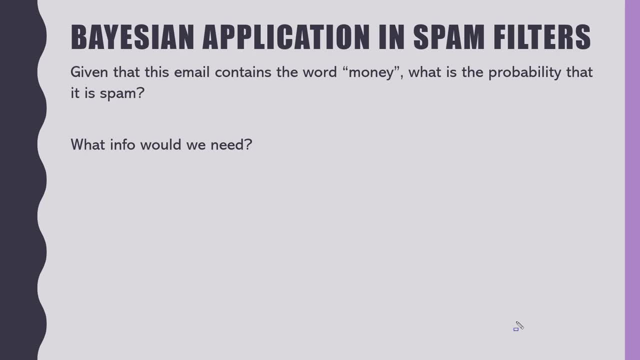 whatever email you're looking at contains the word money, what's the probability that it is spam? I'm not expecting you to answer the question, but I want to know what stuff do you think we would know, would need to know to answer it. So we need to know what percentage of emails have money. 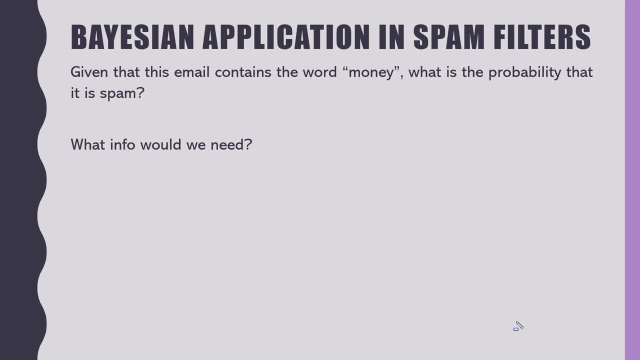 in it. What else would we need to know How many? how much spam does exist? And we don't even necessarily know that number right, Because you might have gotten a spam email and you didn't report it. but based on the data we have, what percentage of all email is spam? 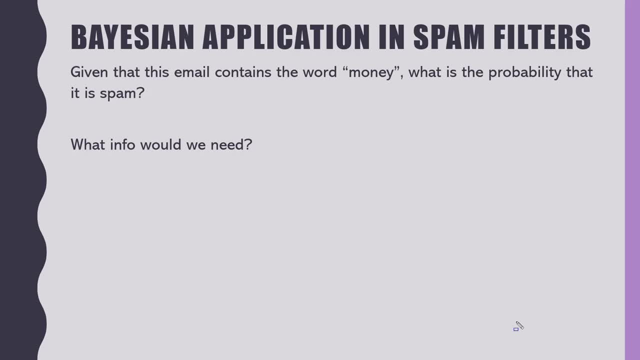 right, Just like you were saying a minute ago, we don't not everybody's taking a cancer test, So the more we, the more people that take it, the more we can update our data. So I'm going to go back and solidly say, yes, that would make a difference. 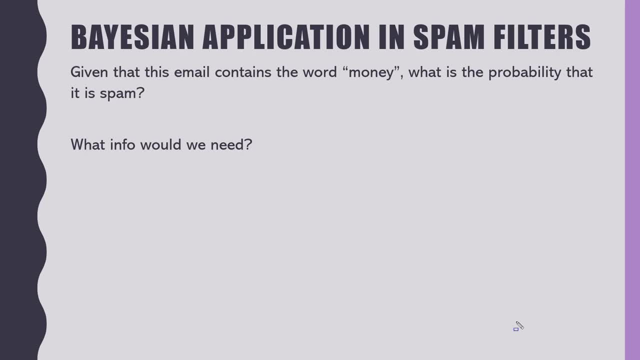 because I originally said it wouldn't, but yeah, it will. So we need to know total number of spam emails that exist based on the data we have, total number of emails that have the word money in it and what percentage of all emails are spam. So we need to know what percentage of all emails 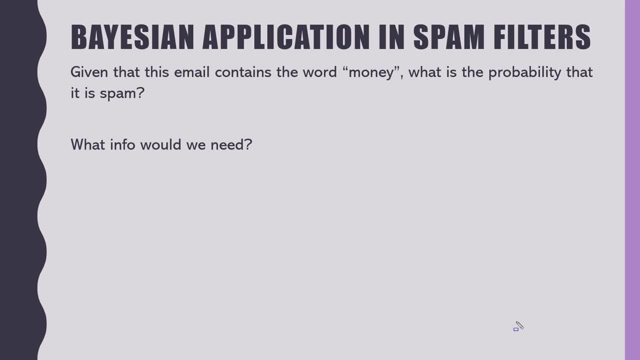 in it Anything else. So probability, that which is total probability, right, of containing the word money, right, Yeah, Probability of a non-spam and a spam having. yeah, So we want to know. non-spam emails: how often do they have the word money and spam emails: how often do they? 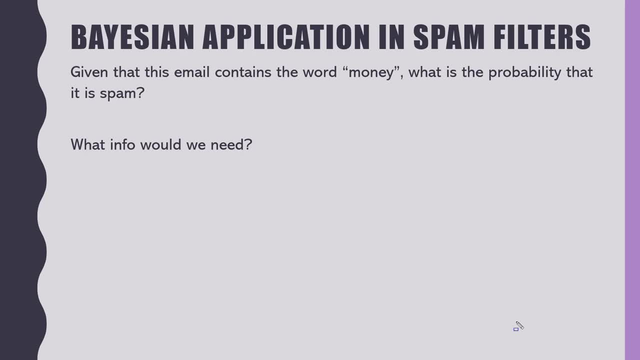 have the word money. That's the data we would need to know to figure out if this one email, whatever that email is, is spam. Now look in the book, in chapter 7, point 3, and it has a whole section on some actual calculations with different keywords. 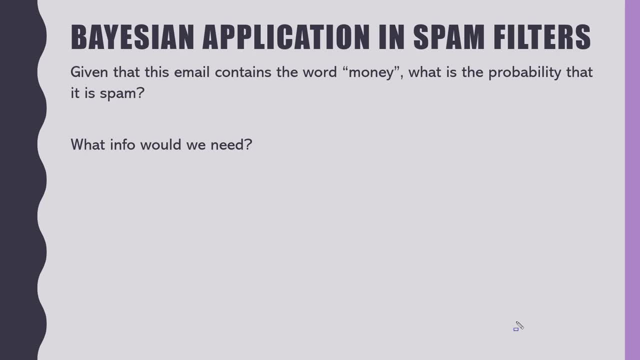 and it has some statistics and some numbers in there. I think Rolex is a popular one. If the word Rolex is in there, it's pretty, it's probably spam, right, But that. take a look at that in the book and read through that. That's like towards the tail end of the chapter. But 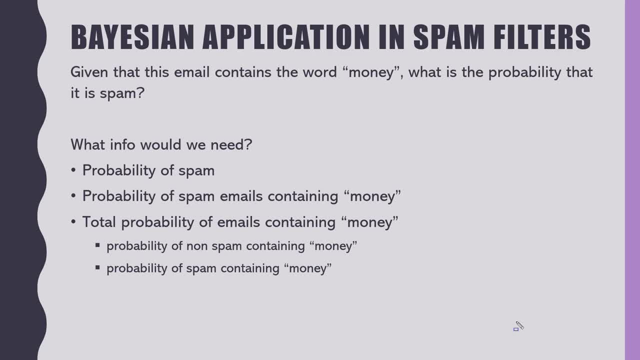 here's the kind of stuff that we would need: Probability of spam and all like, as we mentioned, probability of spam emails containing money, probability of emails containing money which is non-spam and spam, Which is exactly everything we all discovered. If we had that information, we could figure out. 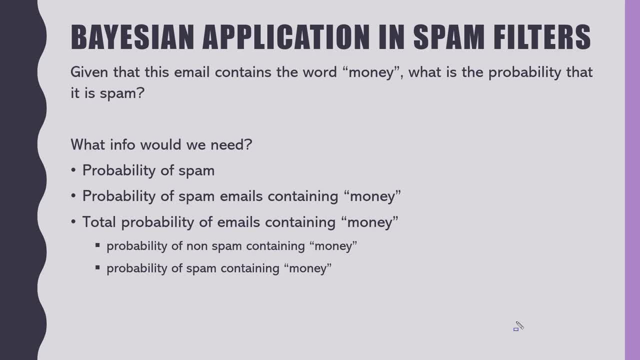 what's the probability that this email is spam? So, even though we're not going to plug any numbers here, what I want to just briefly mention is, conceptually, how would this work If the spam filter software on your server, on an email server, it can read the subject line, or it can. 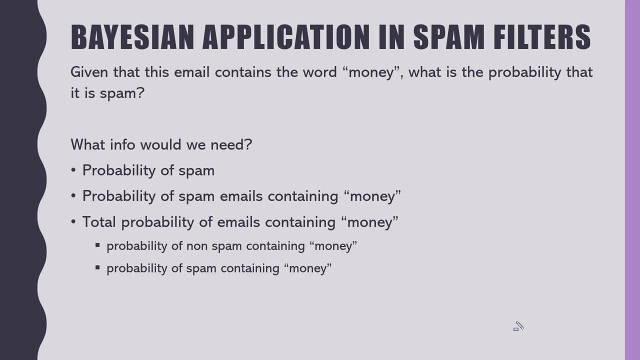 read the email right. You can just have a text parser that can look for text. That's pretty easy. You guys have probably all done that in Java at some point. Okay, so you can parse through the email, look at it and then look for the word money, Or maybe you've got a list of 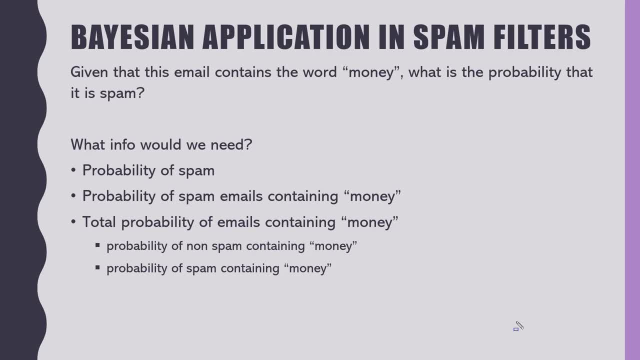 keywords you're searching for and you have data on every one of those. So the word Rolex: We have data and again, I don't know the numbers, but we have data on the word Rolex, how often it appears in all emails, how often it appears in spam emails. We know the probability of spam total. 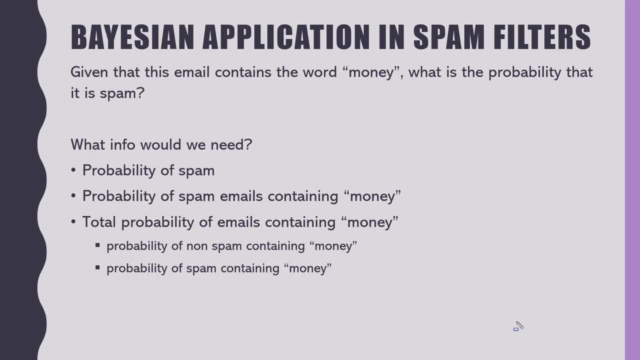 which is going to be the same for no matter what we're looking at. It's just a total probability of getting spam. So this filter can calculate based on the keywords. we're searching for Rolex or anything about dating sites or sex or this kind of stuff. those are 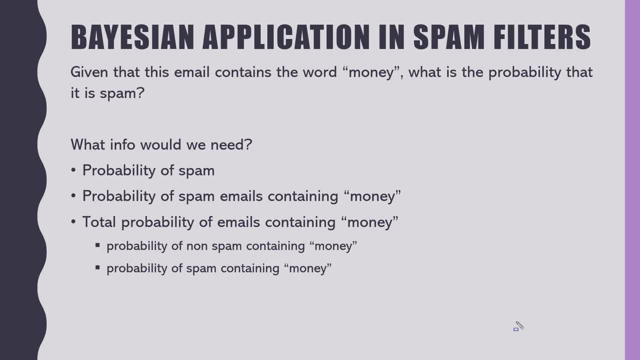 probably all spam. right, Or medicine or this kind of stuff, or money- all of that stuff is probably spam, But the filter can calculate it and you can tweak the settings on a spam filter. I don't know if you've ever manipulated a spam filter, If you've ever worked on a server. 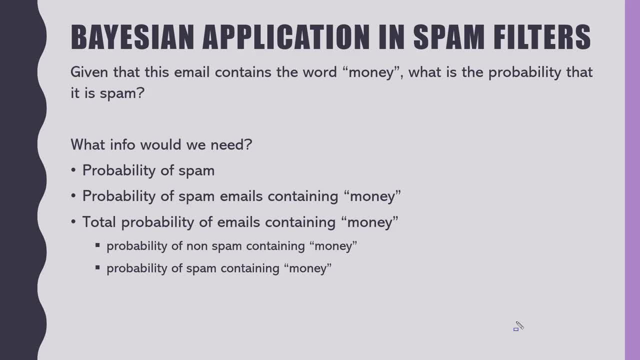 on an email server. you can tweak it to be super sensitive or less sensitive, And all you can just have this filter spit out a number. There's a 10% chance this email spam. Now you, as the administrator of the server. you make a decision. Well, what? 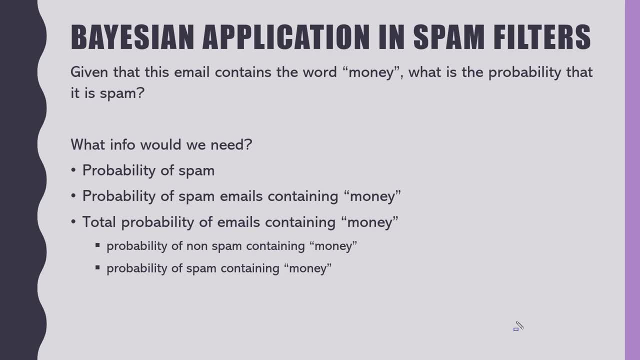 percentage am I willing to risk? If it's a 50% chance that it's spam, should I let it through. If it's a 60% chance, 70% chance, right Maybe. if it's a 10% or less, I'll let it through. 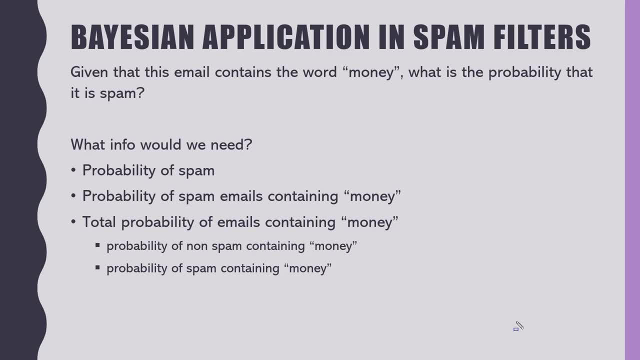